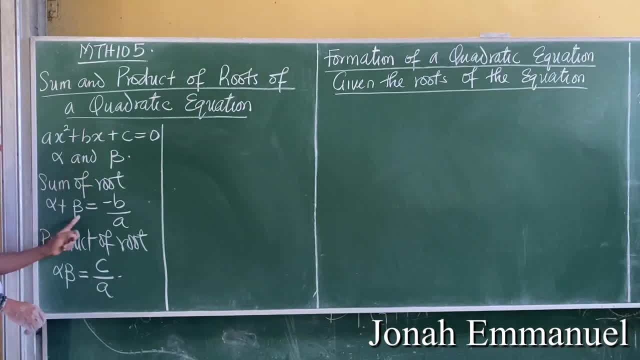 So here's what you should know about it. If I sum my two roots, if I add them up, the value corresponds with negative b over a. If I multiply them- that's alpha times beta- the value corresponds with c all over a. 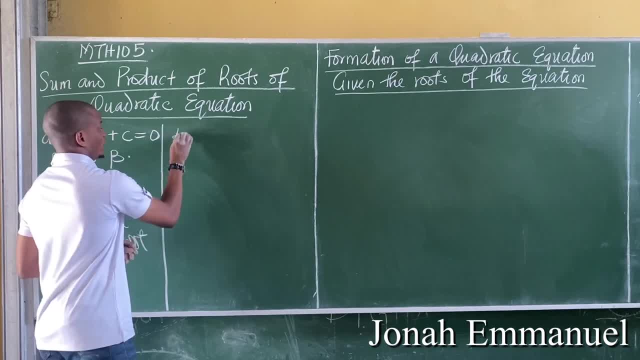 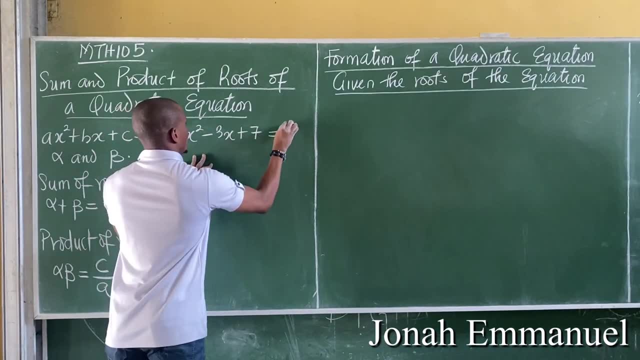 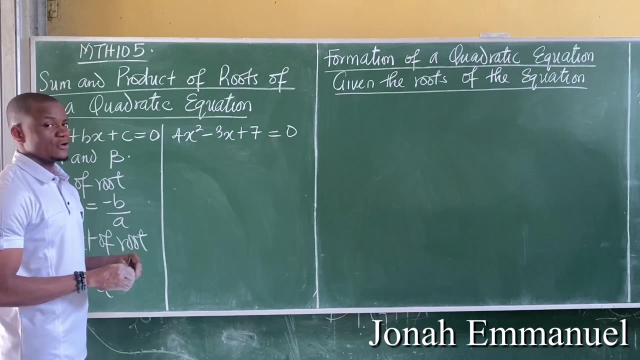 Let's do an example. Let's say I have the product equation 4x squared minus 3x plus 7, equal to zero, And I'm asked to find the sum and product of roots. First of all, how to get the value of a, b and c. 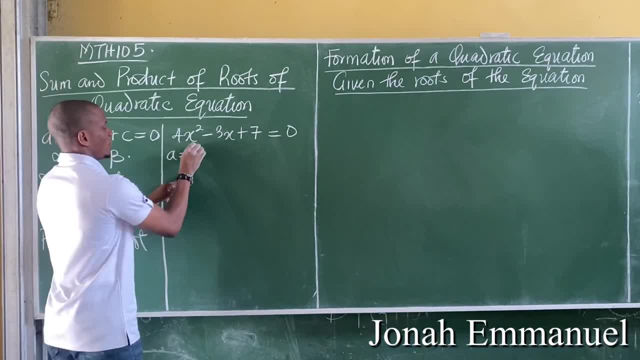 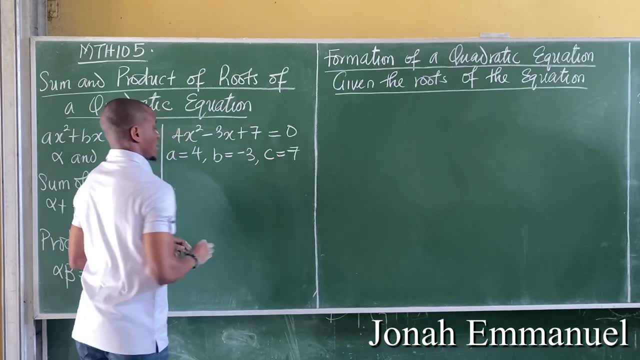 In this case, now, a is equal to 4, b is equal to minus 3, and c is equal to 7.. Let's get the sum. Let's get the sum of roots. Let's assume the roots are alpha and beta. 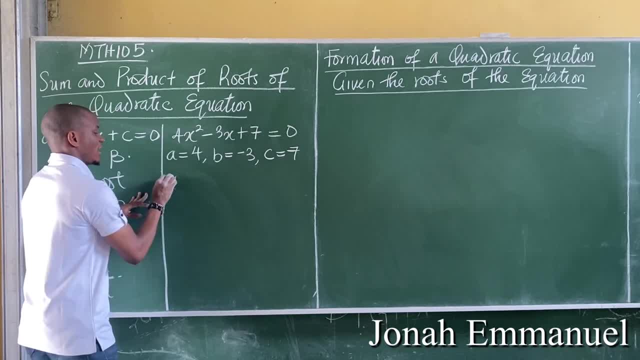 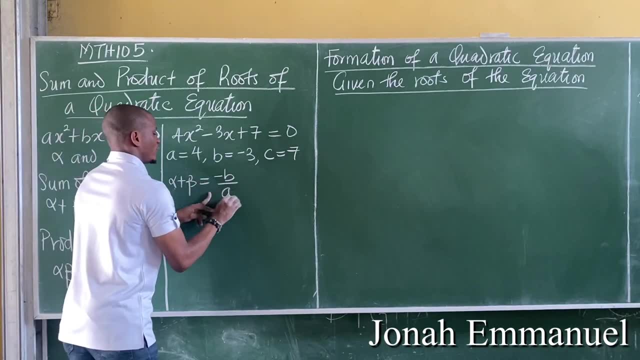 So if my roots are alpha and beta, I will have that sum of roots. alpha plus beta, we said, is equal to minus a over a. That becomes minus b. all over a Impute value becomes minus. b is minus 3, so it becomes minus minus 3. all over a is 4.. 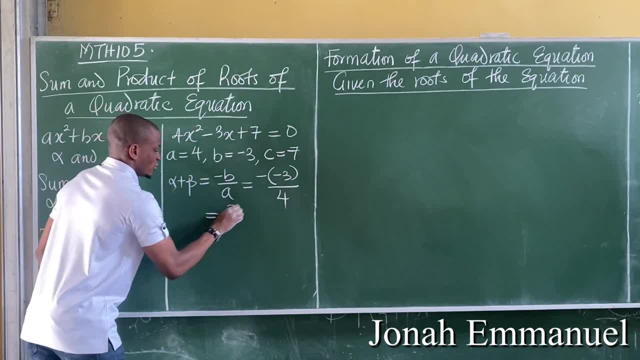 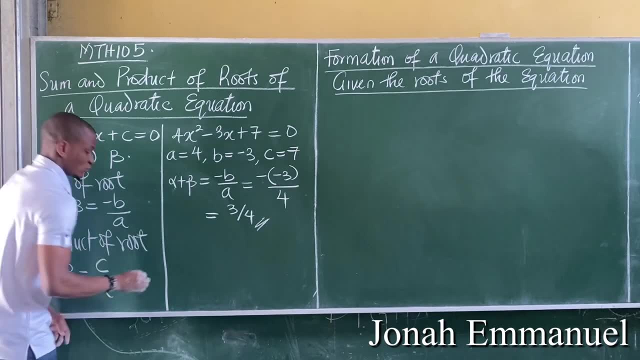 It becomes 4.. This is equal to minus. minus is plus. That gives you 3 over 4.. So if I look at sum of roots, I have 3 over 4.. Let's look at product of roots. Product of roots becomes alpha beta, which we say is equal to c over a. 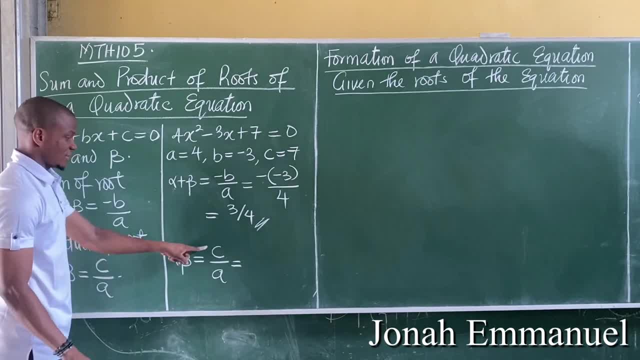 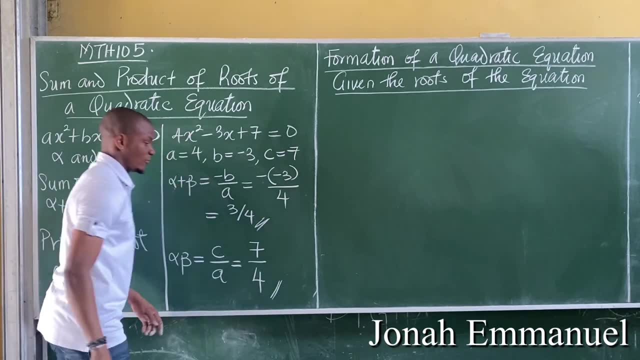 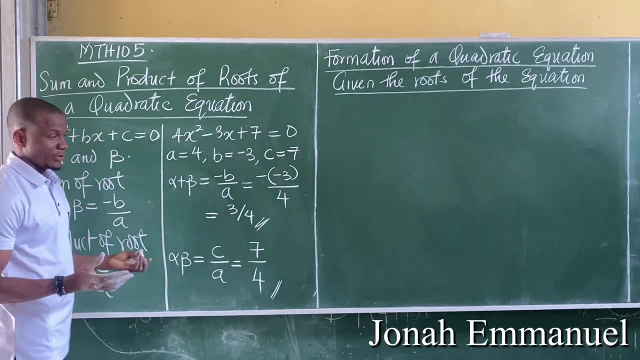 That gives c all over a Impute value. c is 7.. That becomes 7 all over. a is 4.. I'm having 7 all over 4.. Alright, so this is what we mean by the sum and the product of roots of a quadratic equation. 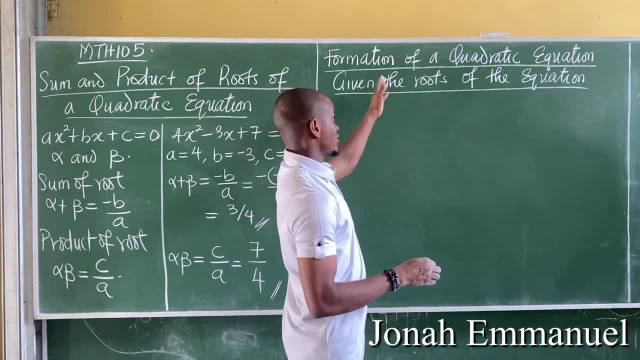 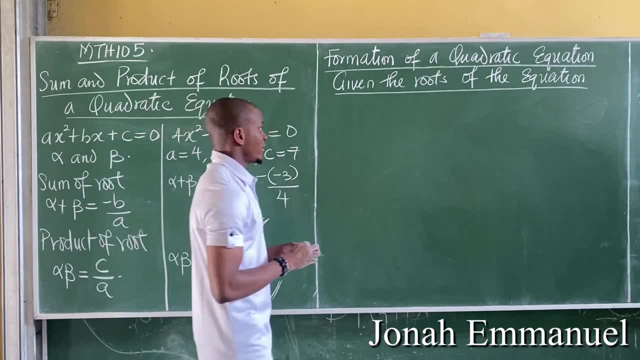 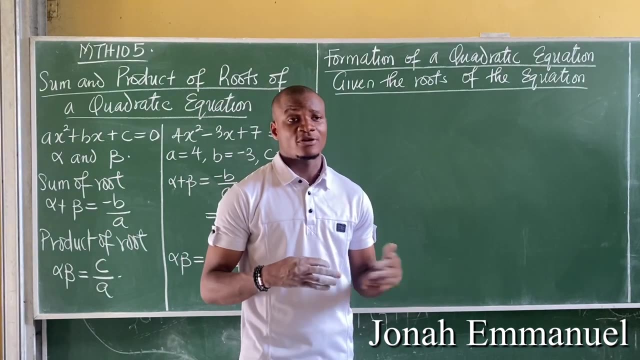 This is how this is done. Alright, let's look at the next concept here: The formation of a quadratic equation. given the roots of that equation, Alright, so let's say: here's what you should note: If I'm given the roots of a quadratic equation, of course I expect that the roots of every quadratic equation should be 2 in number. 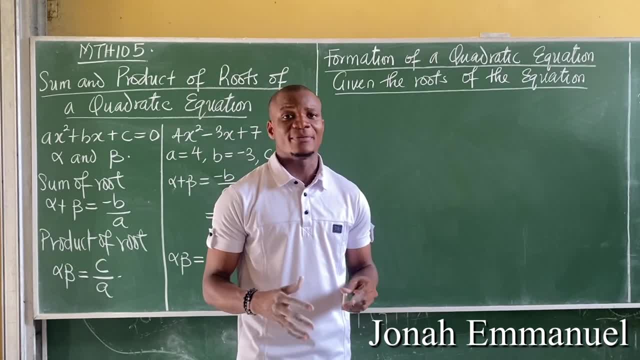 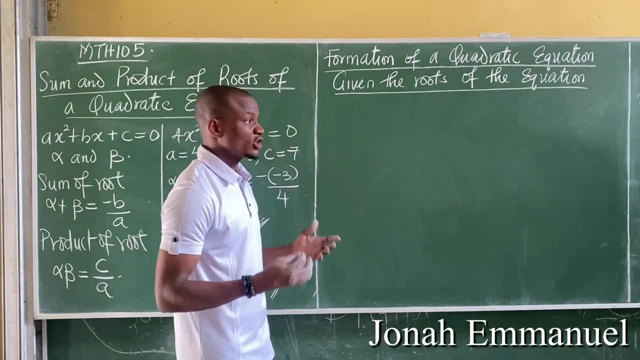 So if I'm given the 2 roots of a quadratic equation and I'm asked to find the equation, or I'm asked to form the equation, what do I do Now? here's what to note For the formation of every quadratic equation, given the roots we have, or it comes in this form: 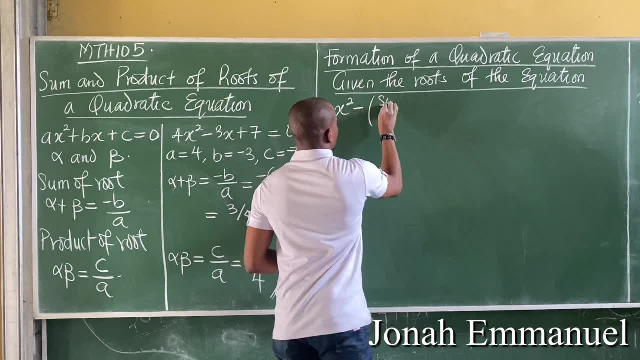 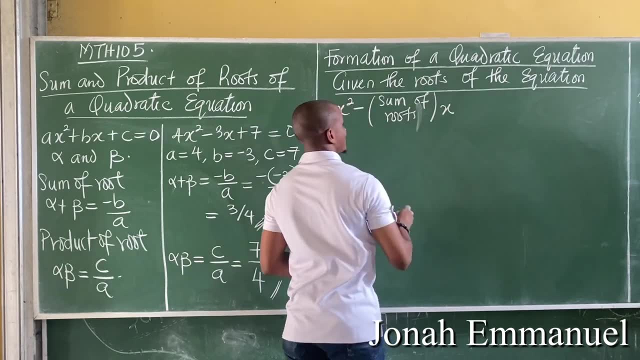 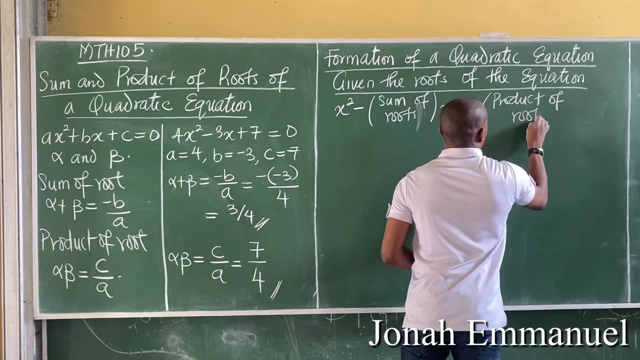 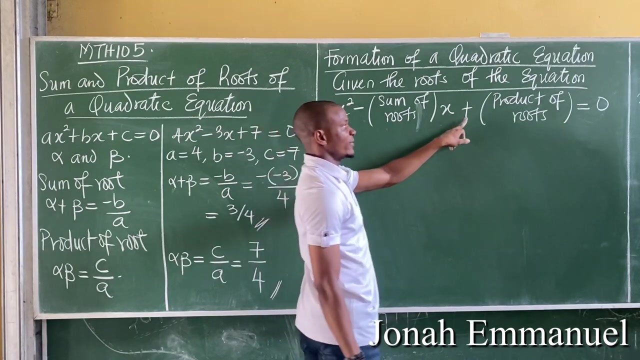 The form is x squared minus the sum of roots. minus sum of roots. multiplying x plus the product, the product of roots is equal to z. Okay So x squared minus sum of roots. So, for instance, x plus product of roots is equal to 0.. 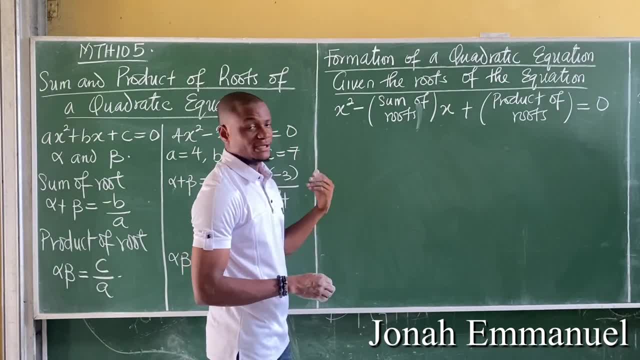 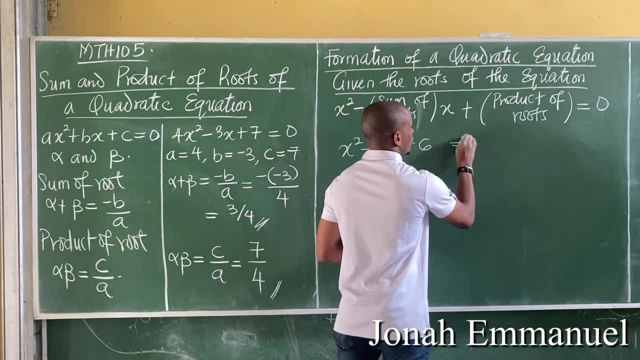 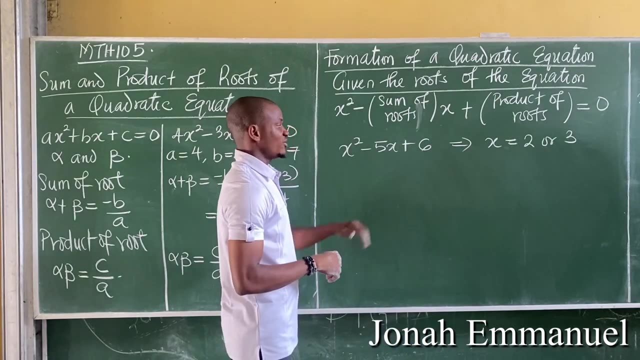 Now, before now, we did an example in our previous classes, Something of x squared minus x plus 6, which, after solving, we got our value as x being equal to 2 of 3.. Right, So let's imagine we did not know the equation. 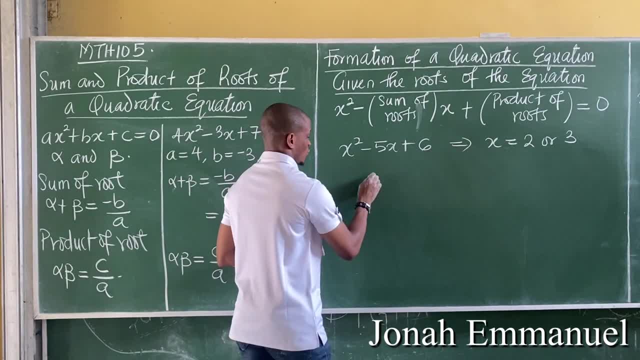 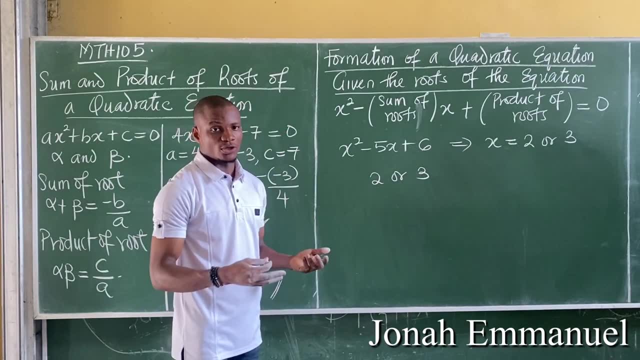 We just had the roots. So we are given the roots of an equation. Let's see Given the roots of an equation 2 or 3.. We are asked to find the equation. What do we do? So in this case? now we are trying to imagine we didn't know. the quadratic equation x equals 0. 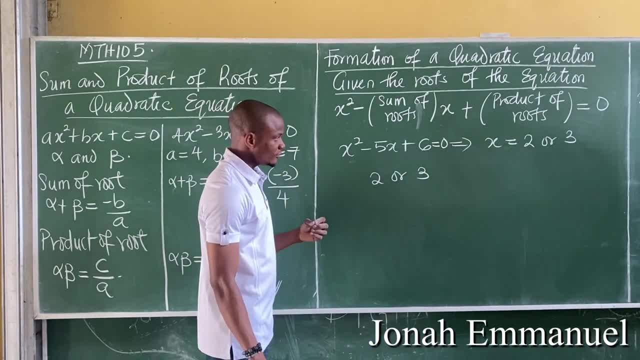 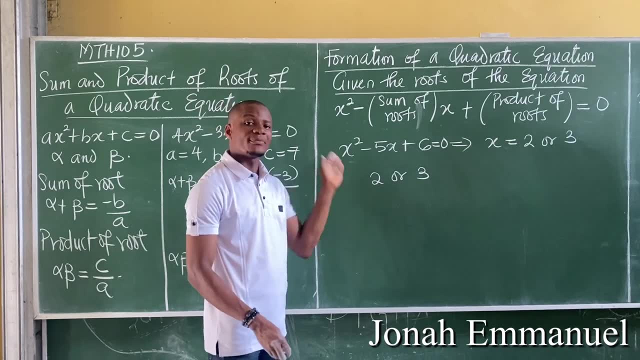 So in this case, now we are trying to imagine what if we never knew the equation, And we are just given just the answers, like this or the roots, And we are asked to form the equation. Is it possible? Yes, it's possible. 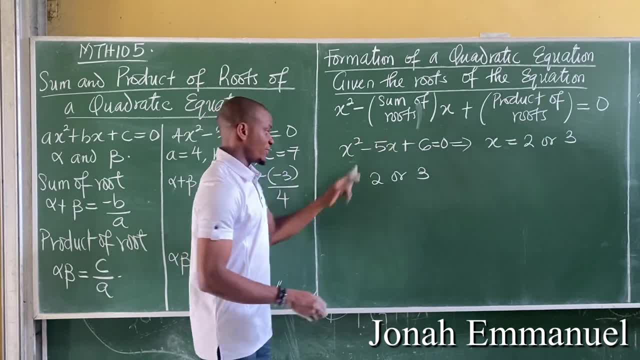 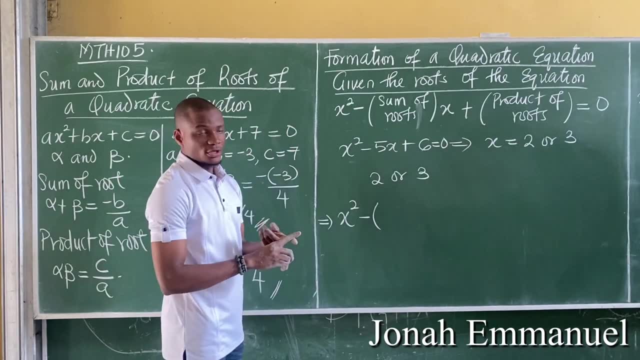 How do we do that? Now? we use this concept From here. now, Forming the equation becomes x squared minus. we set sum of roots. In this case the roots are 2 and 3. So when we say sum, we mean we are adding them. 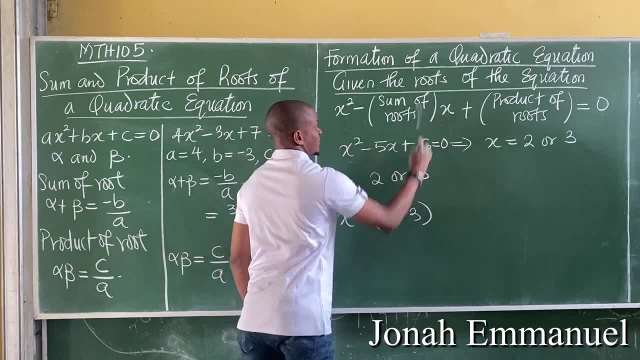 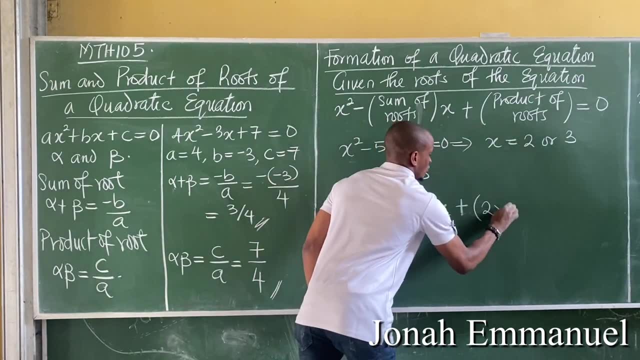 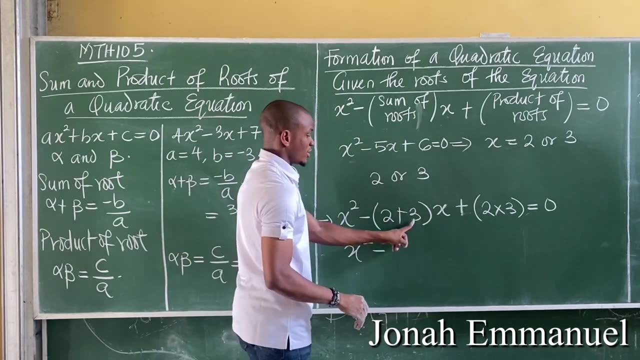 It becomes 2 plus 3, sum of roots then multiplied with x, So that's x plus root of roots. That means I multiplied them, So it becomes: 2 times 3 is equal to 0. This now gives you x squared minus 2 plus 3.. 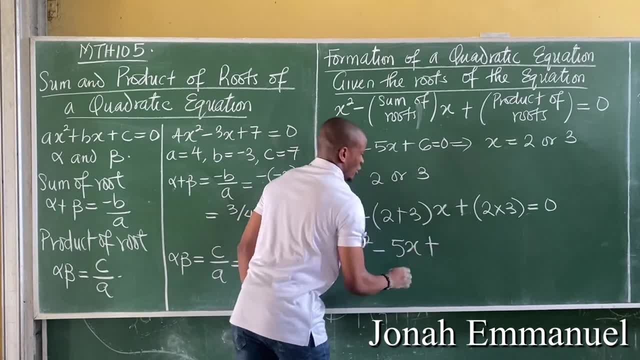 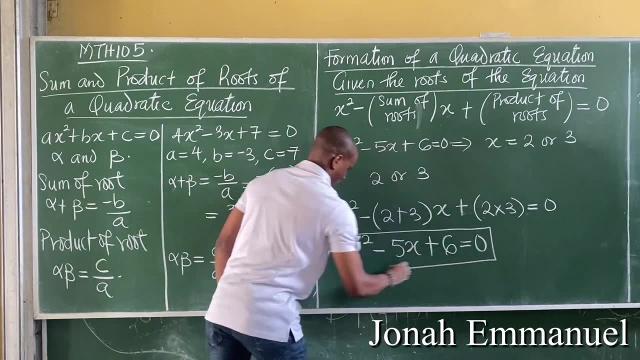 It's 5 times x gives you 5x plus 2 times 3 gives you 6 equal to 0. So I have x squared minus 5x, plus 6 equal to 0.. The same equation from which we got the roots. 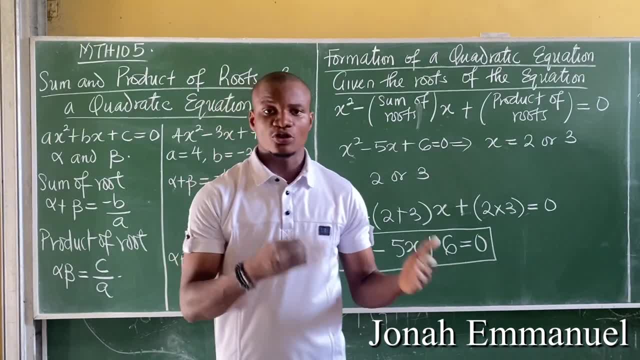 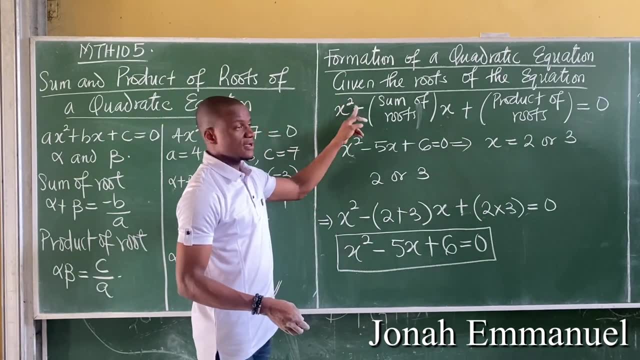 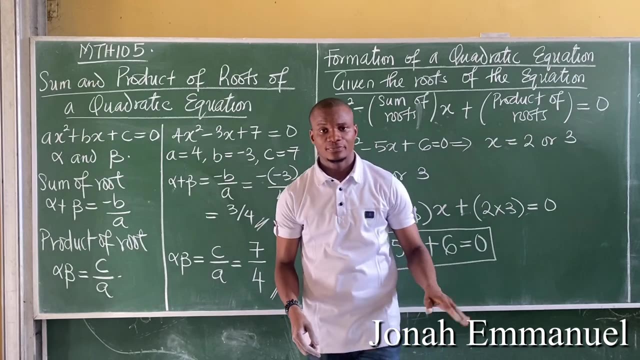 Alright, But the concept is now this: If I'm given the roots of any equation, I can actually form back the equation using the concept of x squared minus sum of roots, x Plus root of roots equal to 0.. Alright, so let's look at this problem. 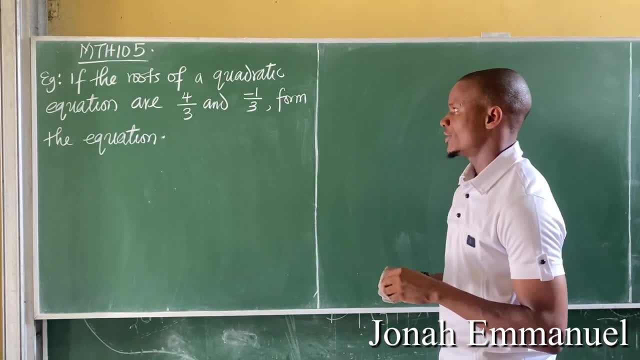 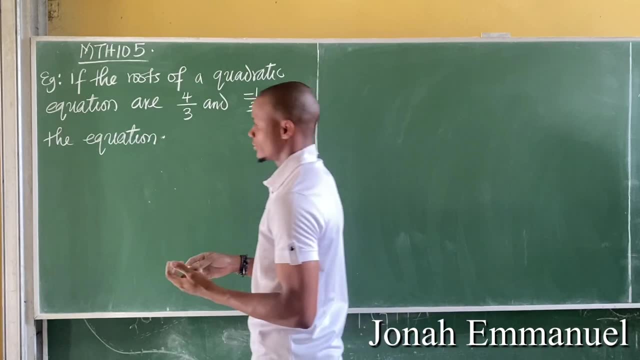 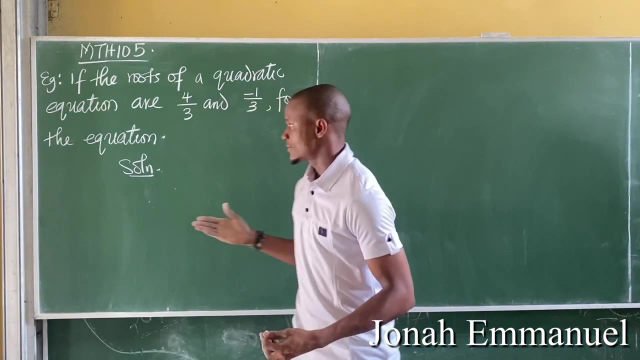 It says that if the roots of the quadratic equation are 4 over 3 and minus 1 over 3. Form the equation Alright In this case. now I'm given 2 roots of an equation, that's 4 over 3 and minus 1 over 3.. 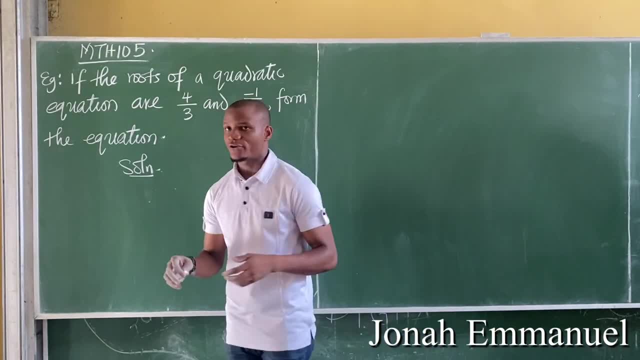 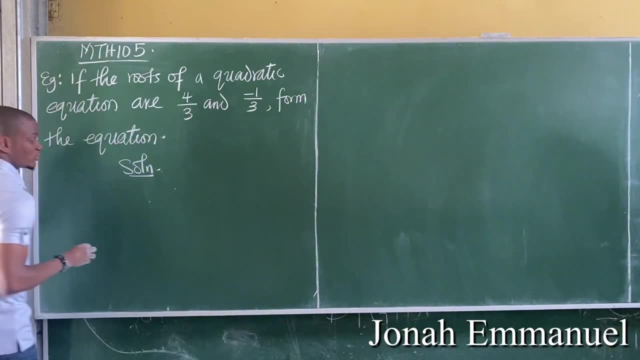 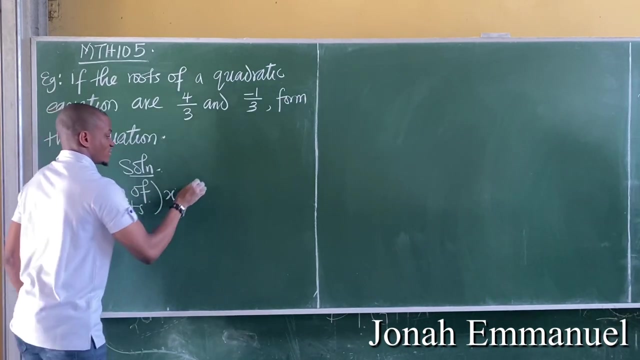 Then I'm asked to form the equation. So how do I do that? First of all, recall the general form for the formation of a quadratic equation. We said, when it comes to forming an equation or a quadratic equation, given the roots, we use the formula x squared minus sum of roots, x plus product x. 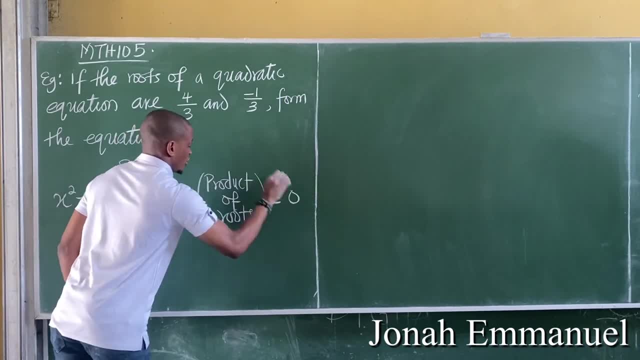 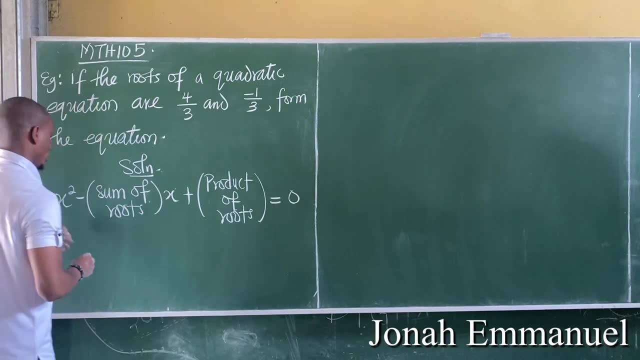 So what I'm going to do is I'm going to take the roots of roots being equal to 0.. Alright, so in this case now, my roots are 4 over 3 and minus 1 over 3.. So this becomes x squared minus. let's add them. 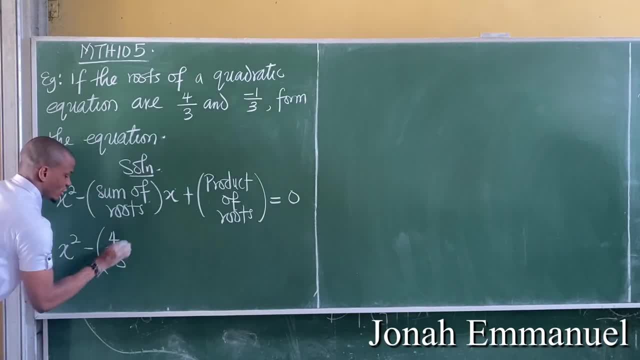 So if I take the sum of the roots, it becomes 4 over 3 plus minus 1 over 3 x plus. if I multiply them taking products, it becomes 4 over 3 times minus 1 over 3.. Alright, 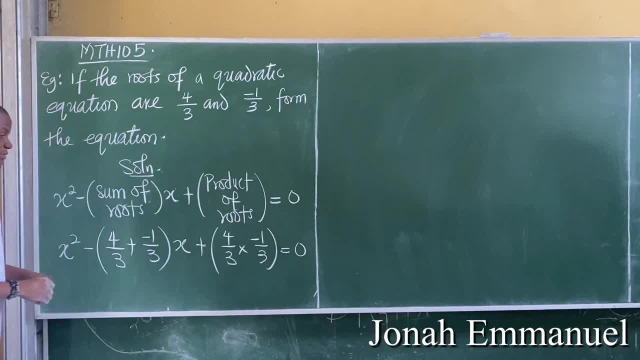 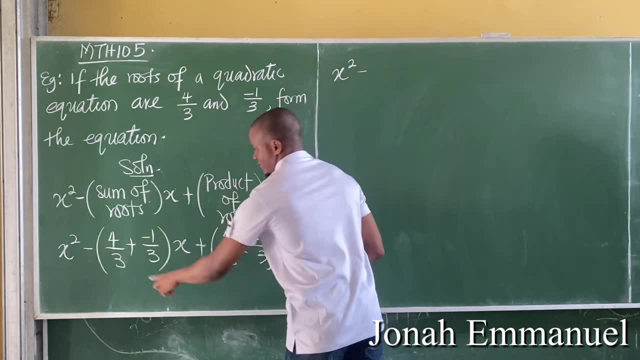 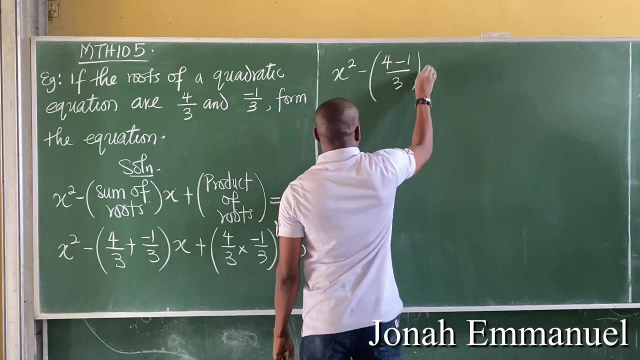 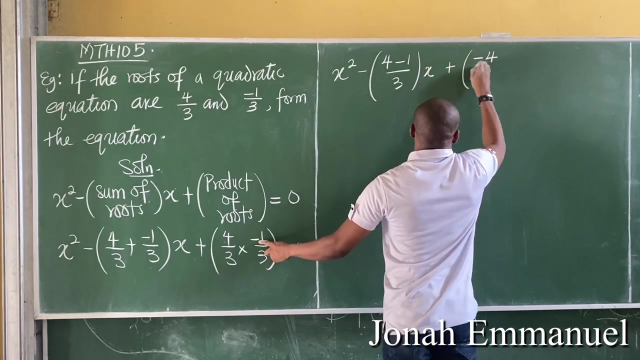 Minus 1 over 3 equals 0. So work this out. We have x squared minus. I'm having the same thing a little. so it becomes 4 plus minus is minus 1 over 3 x plus, and multiplying this 4 times minus 1 is minus 4, all over. 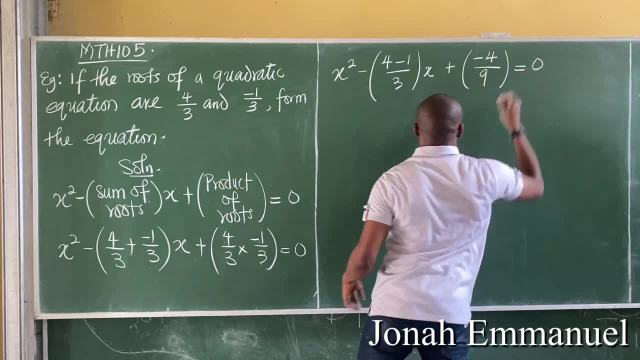 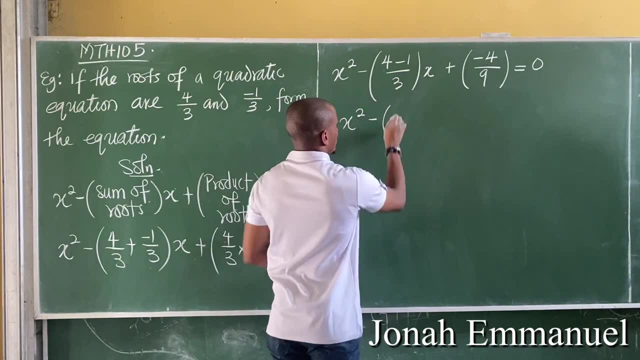 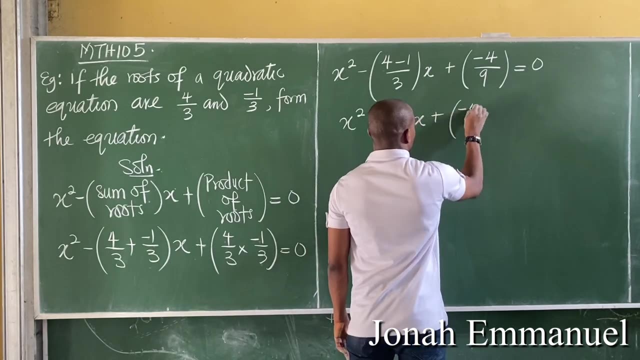 3 times 3 is 9.. That's being equal to 0.. If I work this out, this becomes: x squared minus 4 minus 1 gives 3 over 3 into x plus. this now gives minus 4 over 9 is equal to 0.. 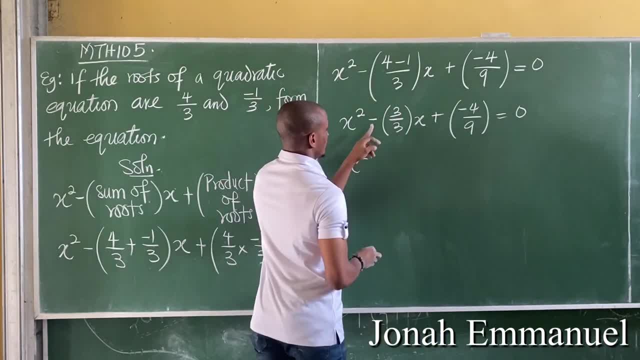 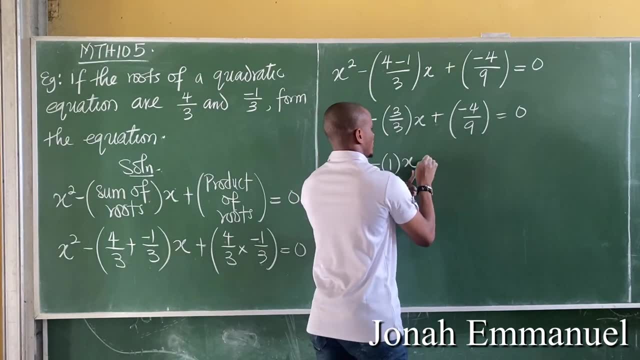 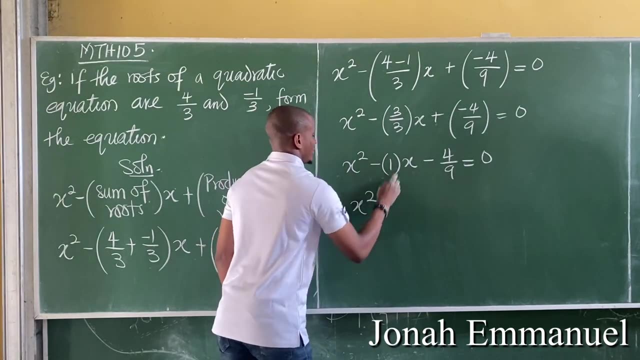 From this I have: x squared minus 3 over 3 is 1,, of course, times x plus minus is minus 4 over 9.. So I have this as: x squared 1 times x, of course, is x minus 1 times x is minus x. 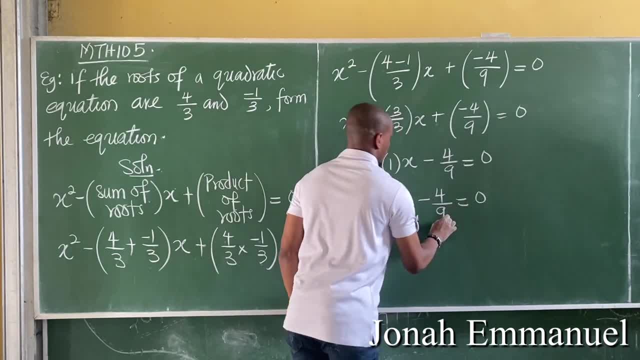 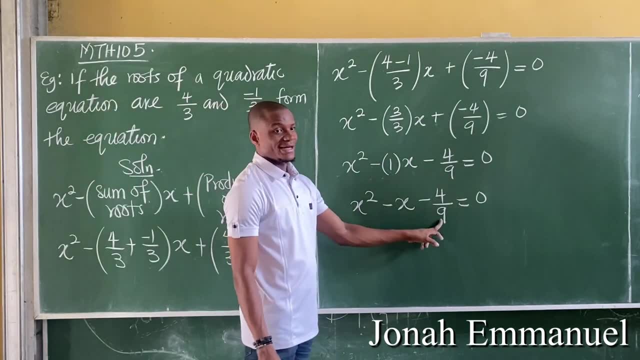 minus 4 over 9 is equal to 0.. At this point you are correct. But the proper form would now be to. since I'm having 9 here as denominator, here I'll have to multiply 2 by 9.. 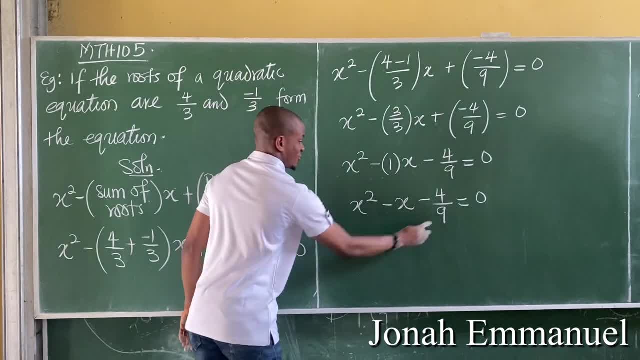 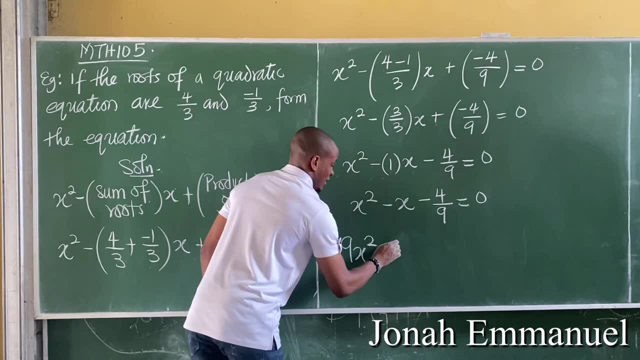 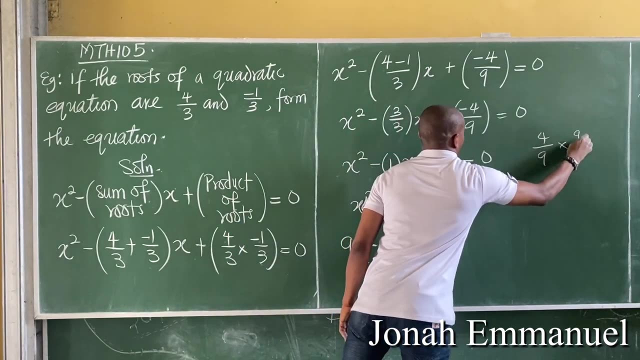 Alright, So that this will cancel out. If I multiply 2 by this, which is 9.. 9 times x squared gives you 9x. squared minus 9 times x gives 9x. This now becomes minus 4 over 9 times 9.. 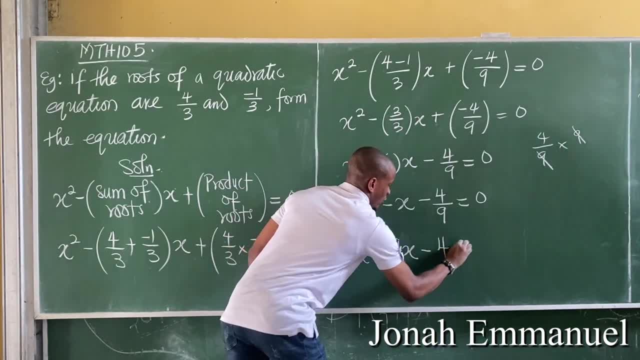 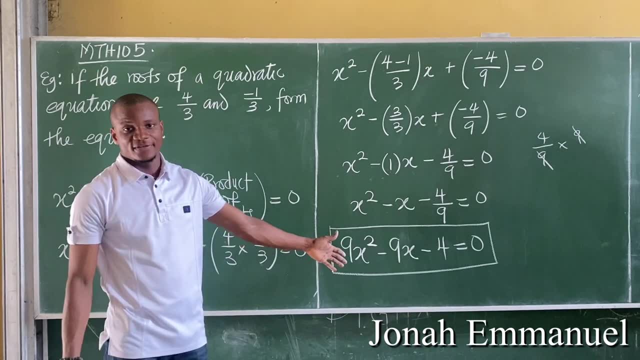 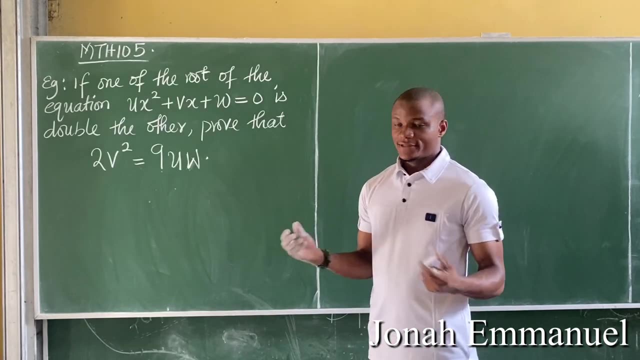 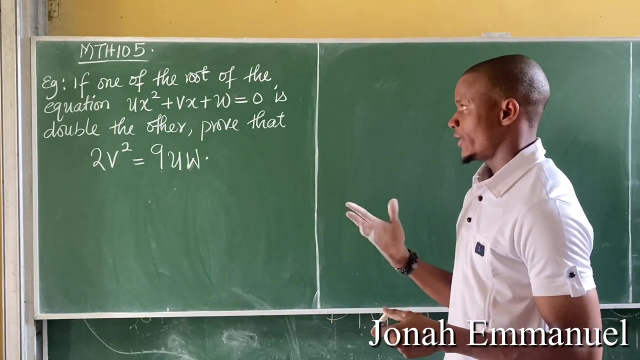 This starts with an ameliorative form. so minus 4 is equal to 0.. This becomes the most proper form of the equation. So I have this as my answer, after simplifying. Alright, let's look at this example. It says: if one of the roots of the equation, ux squared plus vx plus w is equal to 0, is: 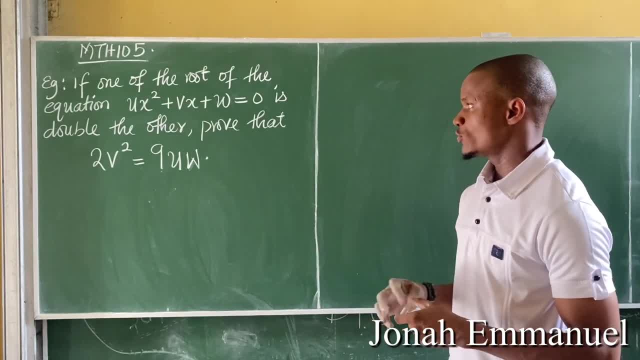 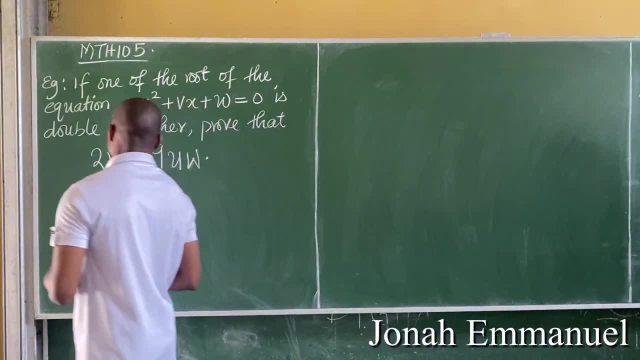 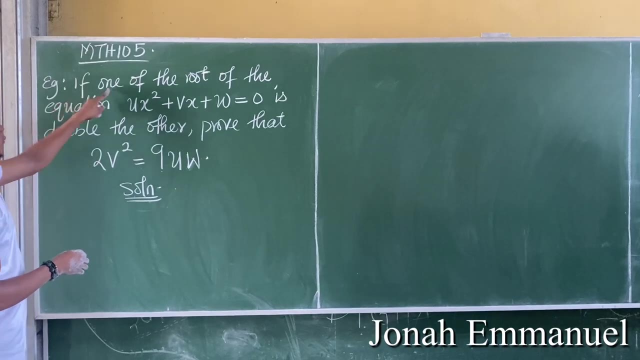 double the order. Prove that 2v squared is equal to 9uw. Okay, so how do we solve this solution? So the answer to the question is this. The answer to the question is this: If one of the roots alright is, double the order. 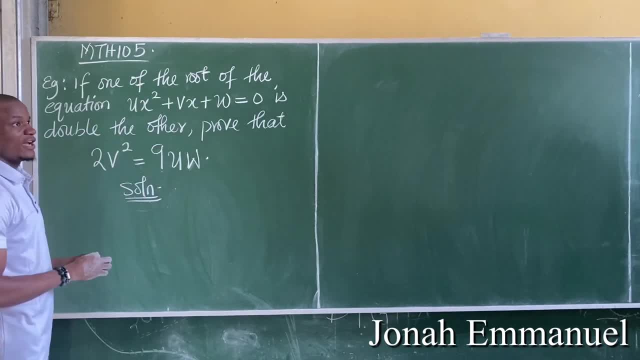 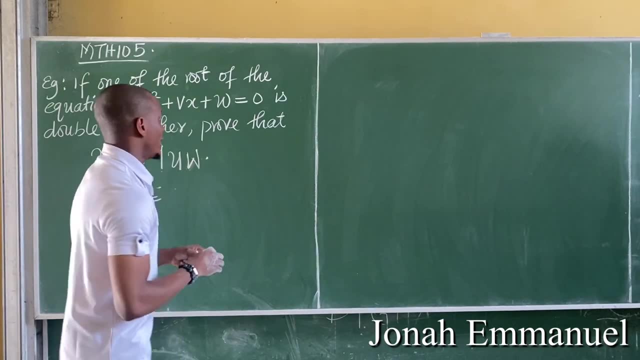 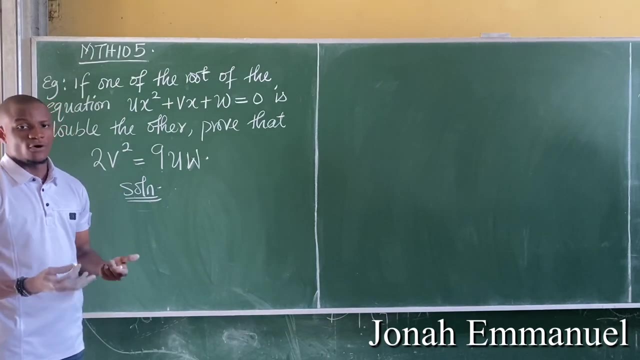 If one of the roots is double the order, Alright. so I have 2 roots there. Now for my 2 roots. they said one of the roots is double the order, Alright. How do you write double the order? How do we express double the order in mathematical form? 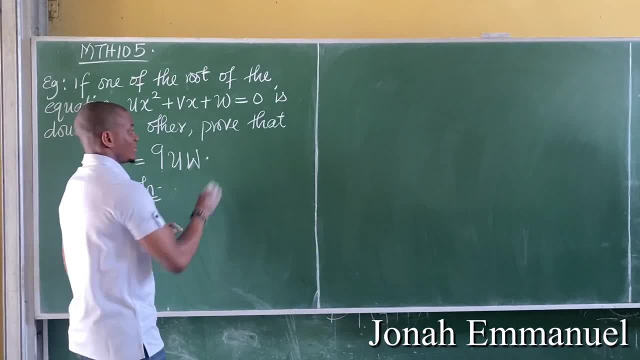 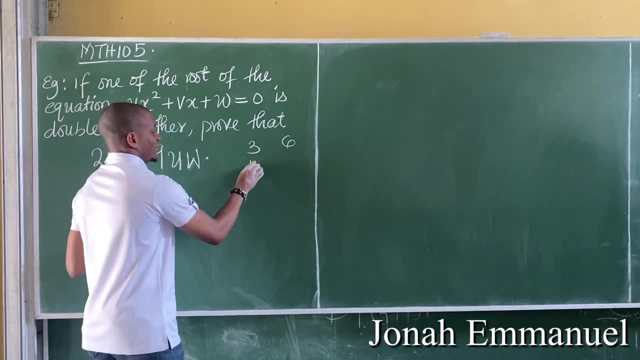 Now let's look at this way: If I have 3,, for instance, Double of 3, obviously is 6.. If I have 10,, for instance, Double of 10 is 20.. So the concept is this. 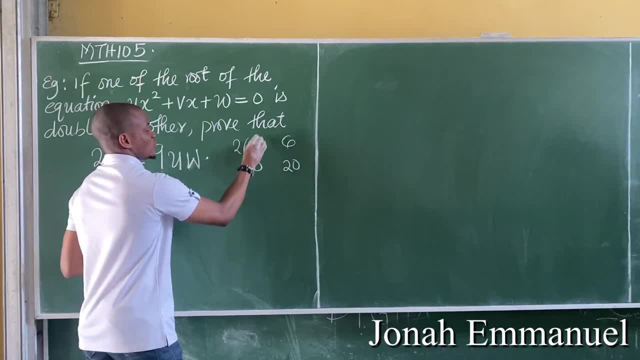 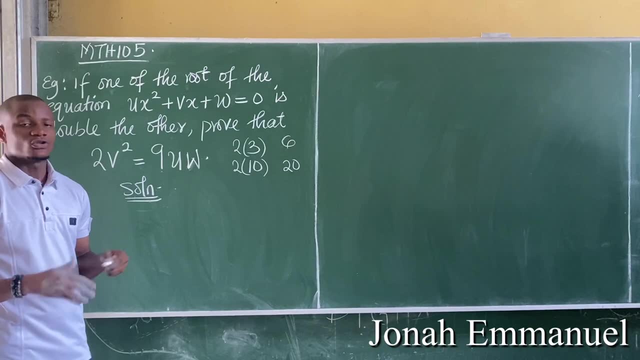 If I'm doubling a number, it means I'm multiplying it by 2.. Okay, 2 times 3 is 6.. 2 times 10 is 20.. So to double a number means to multiply it by 2.. It's a mathematical concept. 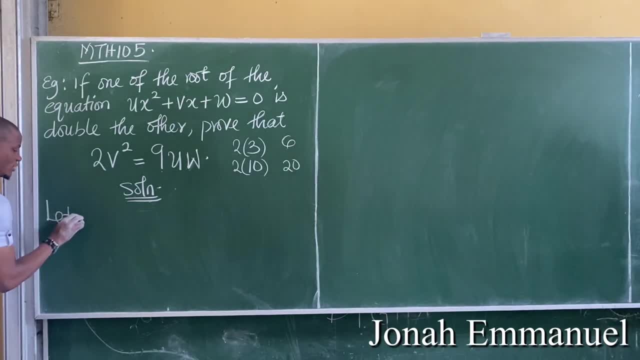 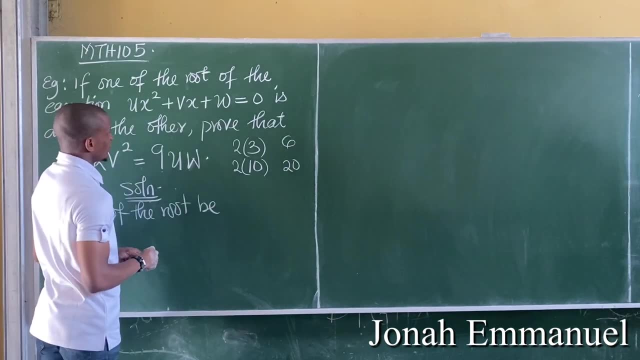 So let's say, let one of the roots. Let one of the roots, Let's say any alphabet We could use: alpha, Let it be alpha. Then the second root, The next root, or the second root, Or the other root, perhaps. 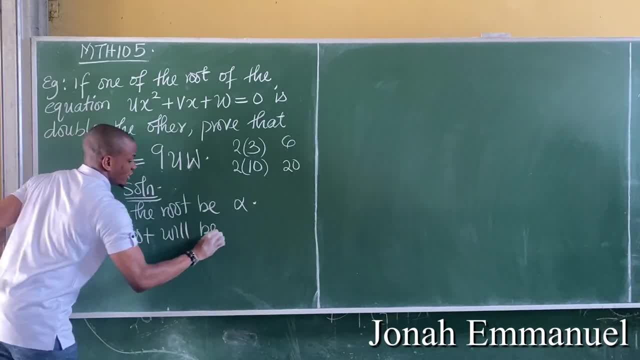 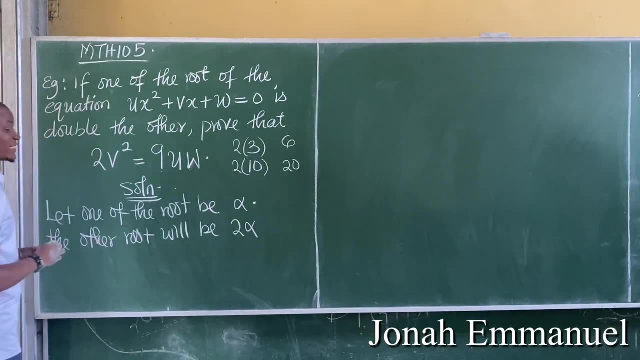 The other root will be 2 alpha. Why Double the first one, 2 alpha. Alright, let's look at the sum of roots. The sum of roots is equal to alpha plus second root there, That's 2 alpha. This will be equal to the set minus b. 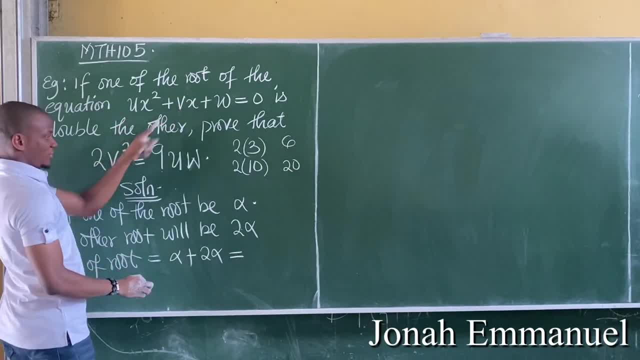 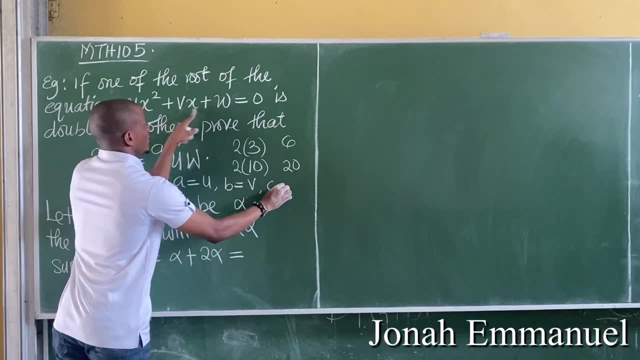 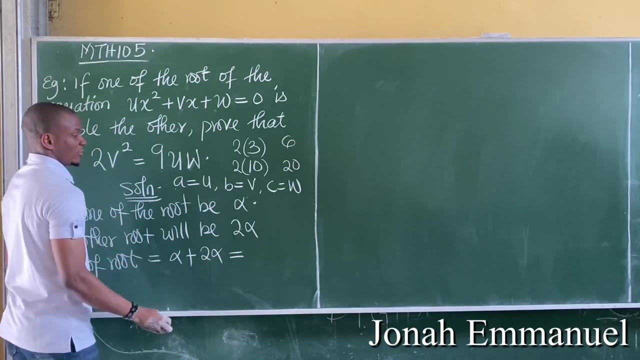 In this case, b is b, Alright, so a is u, Okay. a in this case is u, b in this case is v And c in this case is w- Alright. So sum of roots: alpha plus the second root there is equal to minus b. 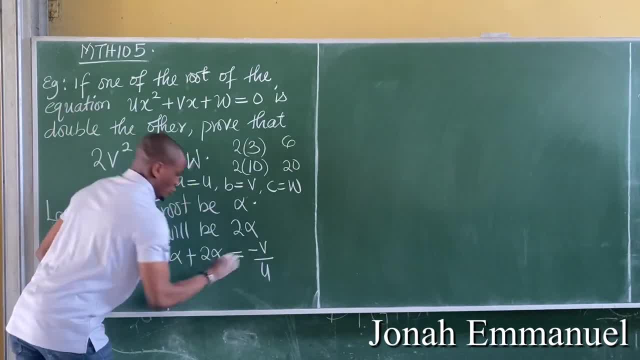 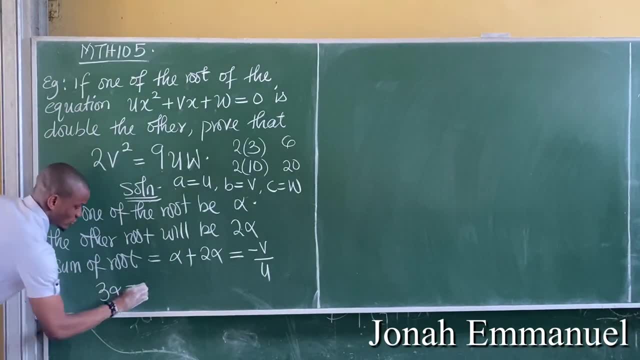 That's v All over a. That's u. If I work on this, alpha plus 2 alpha gives you 3. alpha is equal to minus v all over u. I have this. Alright, let's make alpha subject of the formula. 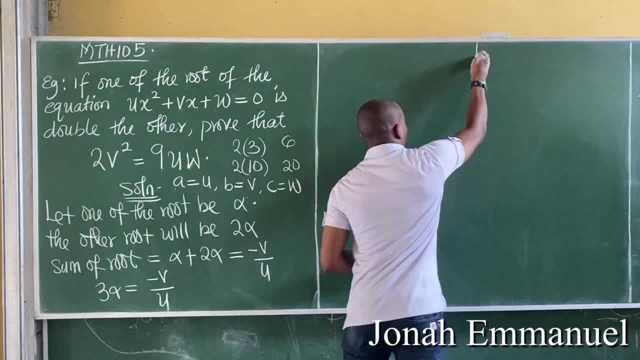 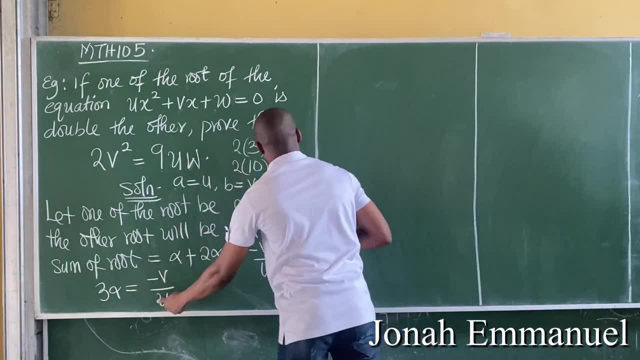 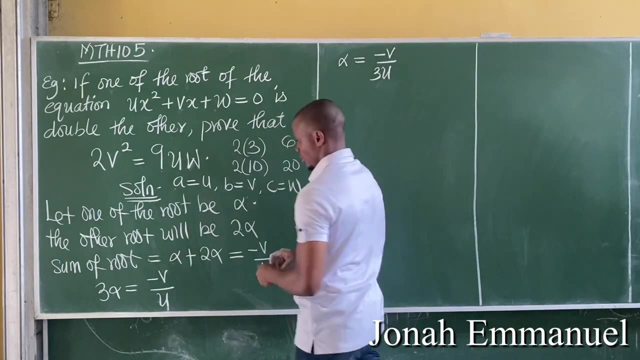 To make alpha subject of the formula. To make alpha subject of the formula, I'll simply move 3 over here. So I'll have that alpha is equal to minus v over u Or perhaps 3u. Simply move 3 over here. 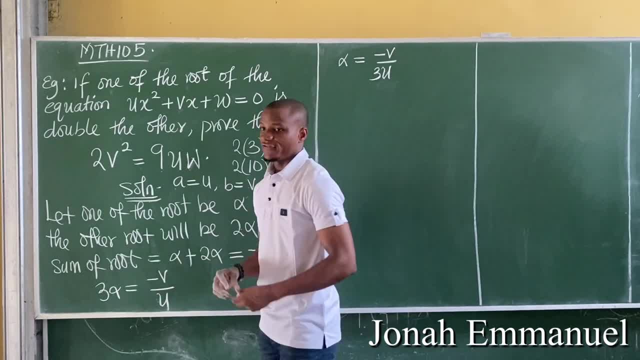 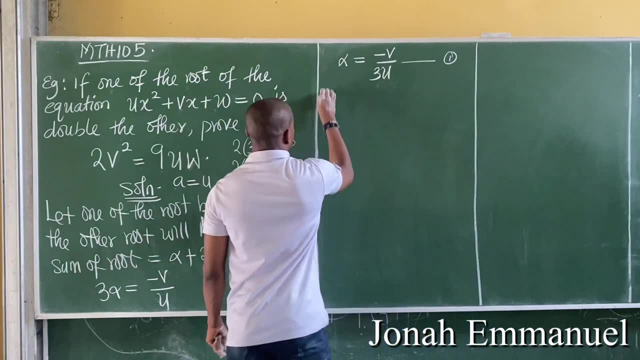 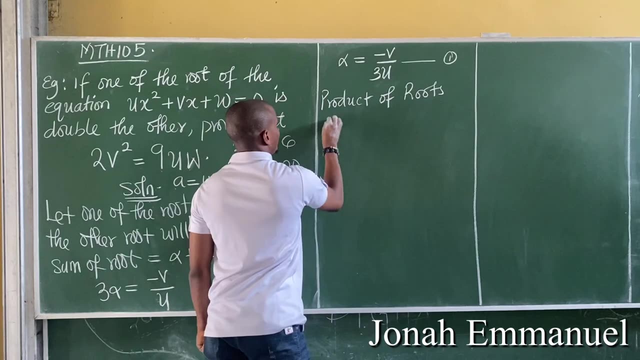 That must be correct. Or you can say: divide both sides by 3.. If you divide both sides by 3, you have this. Call this your first equation. We've gotten sum of roots. Let's do product of roots. The product of roots will now be alpha multiplying the second root. 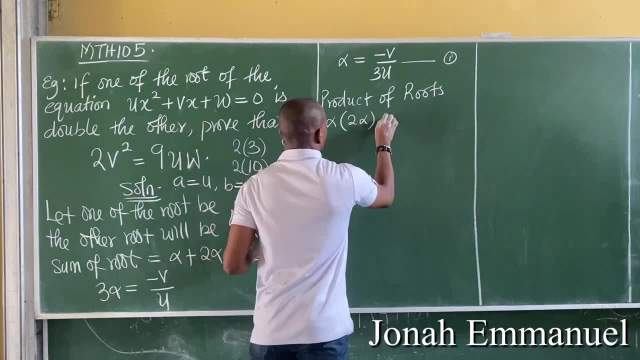 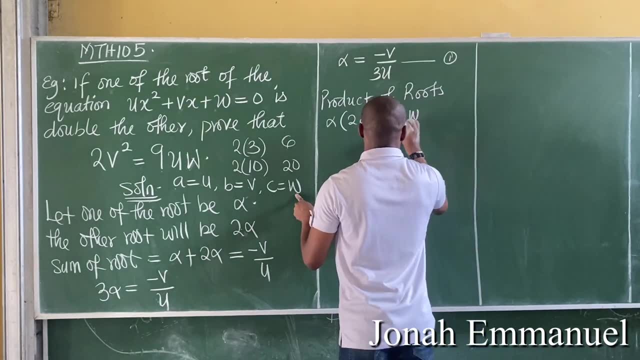 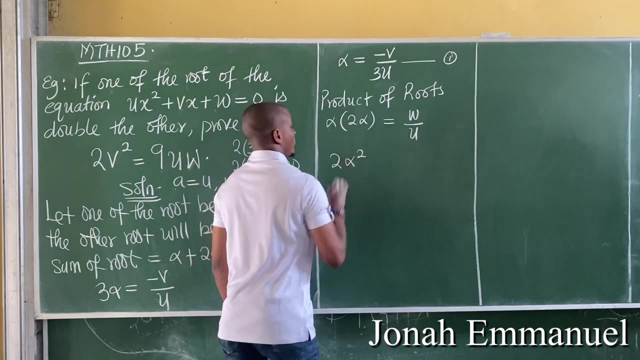 That's alpha multiplying 2 alpha And will be equal to. we said product of roots is equal to c over a. c here is w All over a is u What this alpha alpha times 2 alpha gives you. 2 alpha squared is equal to w. 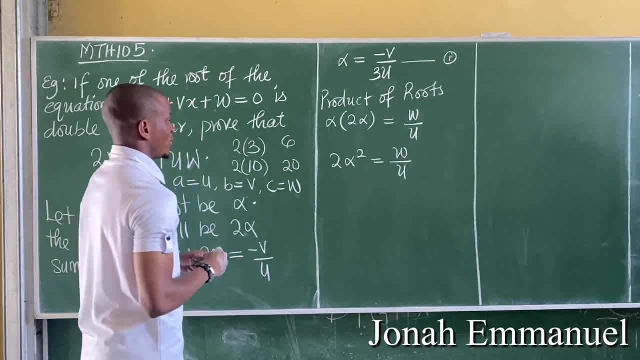 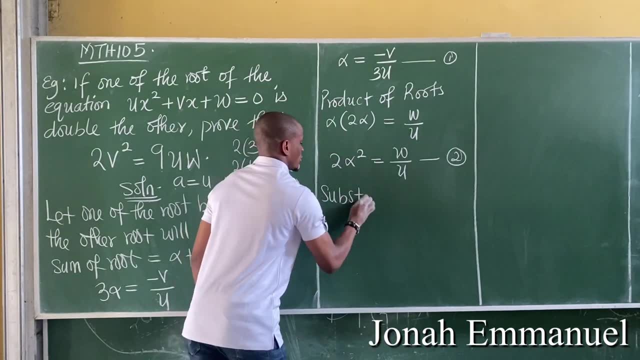 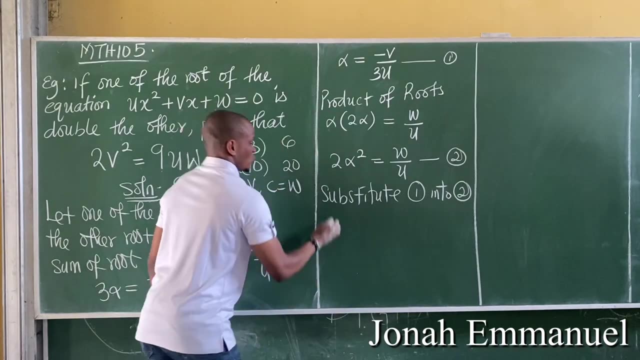 All over u At this point. now you can choose to call this equation 2.. You can choose to substitute. You can substitute equation 1 into equation 2.. From equation 2, I have 2 alpha squared equal to w over u. 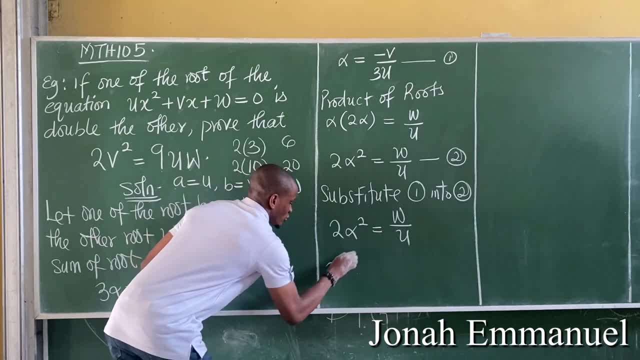 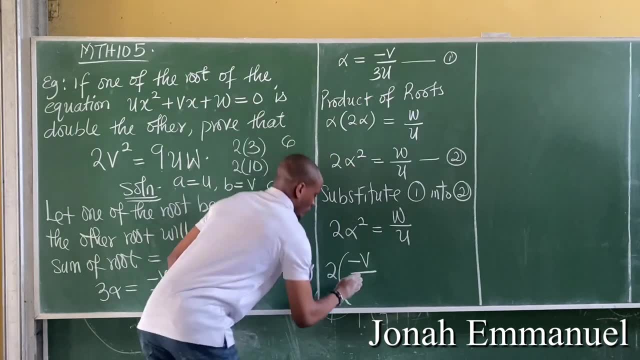 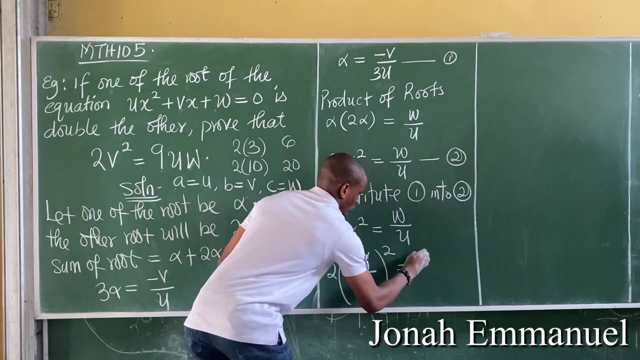 Put the value of alpha there. So I have 2 into what's alpha. Alpha is minus v, minus v, all over 3u, All over 3u. So this is alpha, all squared. All squared is equal to w, all over u. 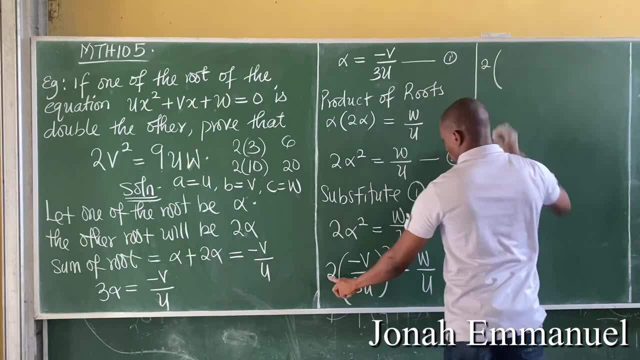 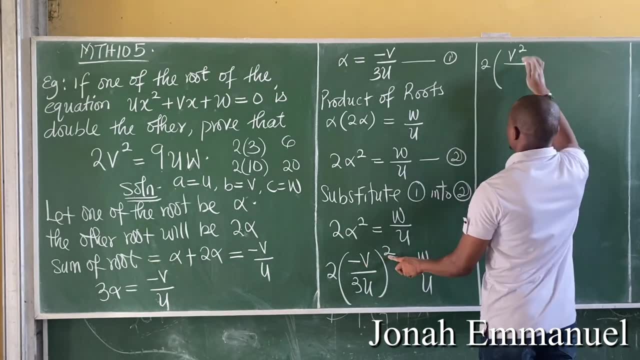 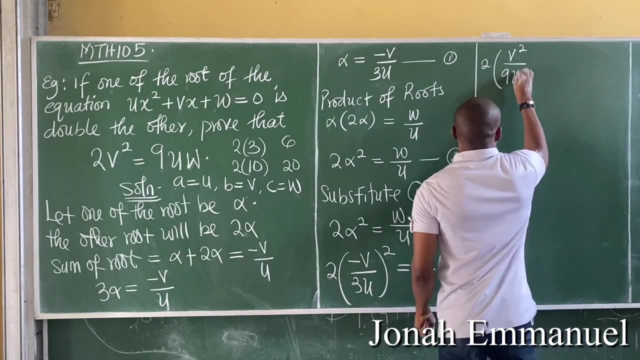 Work this out. This becomes 2 into minus v. all squared gives you v squared. So minus squared gives you positive v squared. we have v squared. Next up v squared gives 9.. Next up u squared, I have u squared. 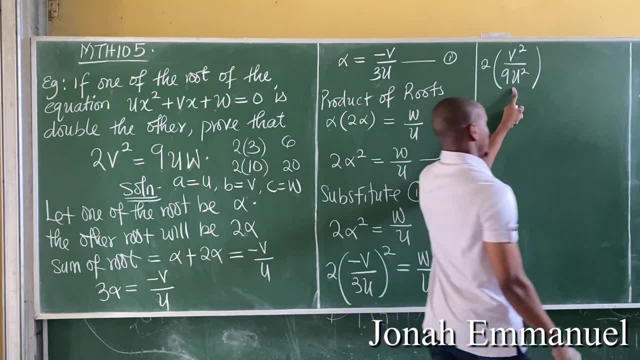 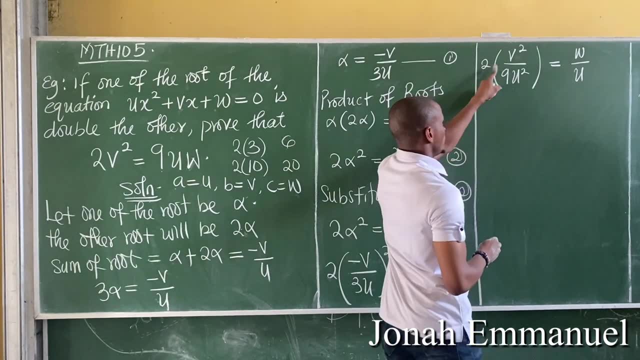 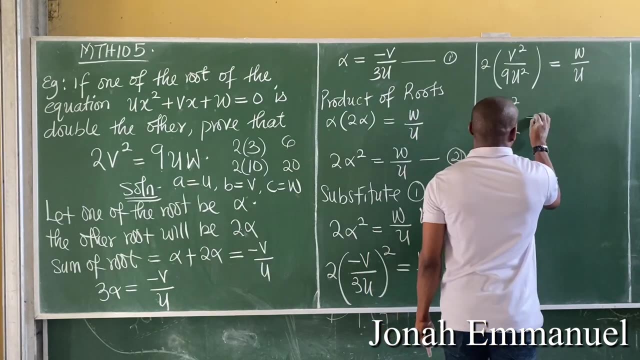 All right. So if I square this you now have this is equal to w all over u. So I have this. Of course, 2 multiplied there gives you 2v squared all over 9u. squared is equal to w all over u. 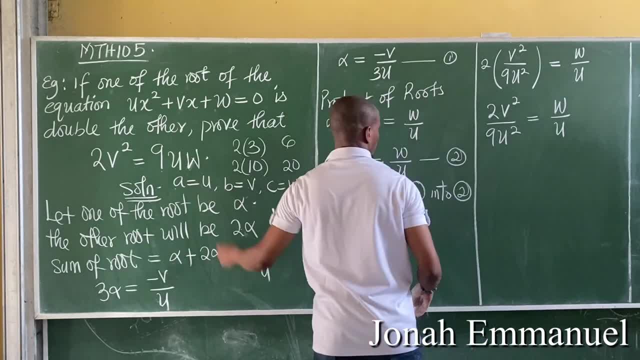 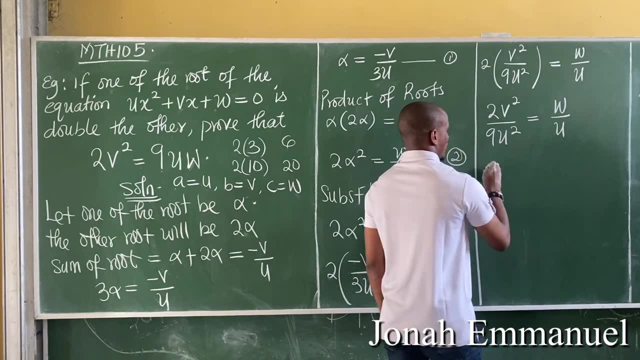 My next task will now be: I will express this in this form, I will move this over here. So cross multiply. This one goes this way. This goes this way. If I cross multiply, it comes 2v squared times u. 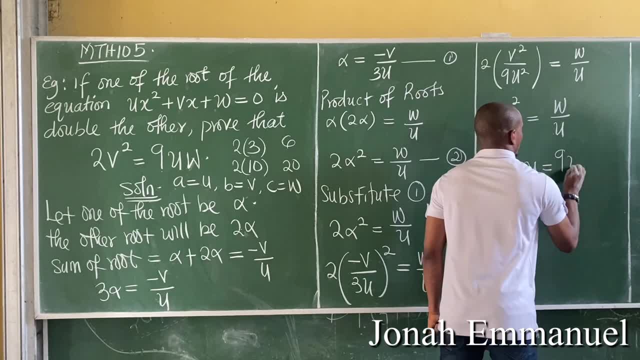 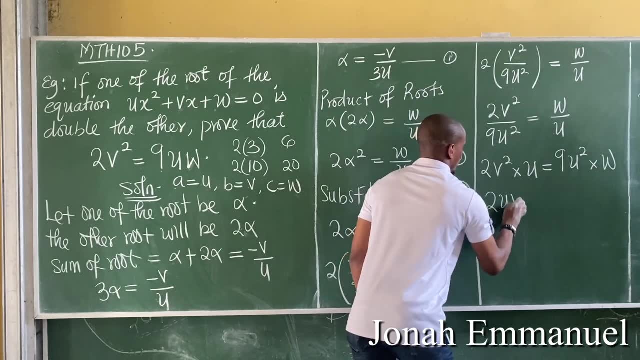 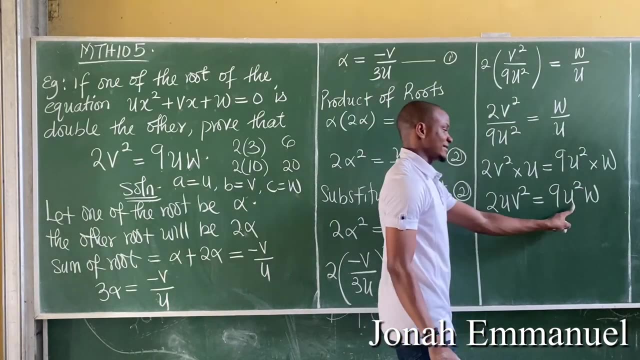 This times this is equal to 9u squared times w. This now gives you 2uv squared is equal to 9u squared w. I can see u here. They are both common to the left hand side and right hand side, So divide here by u. 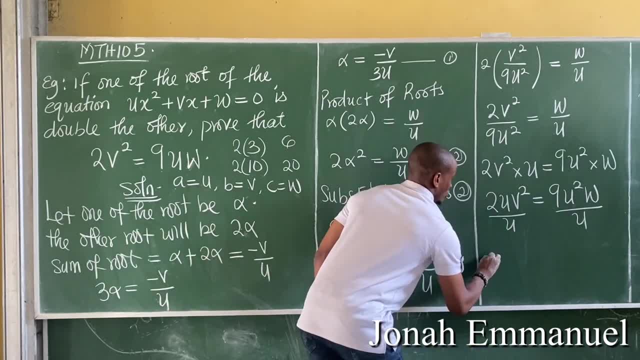 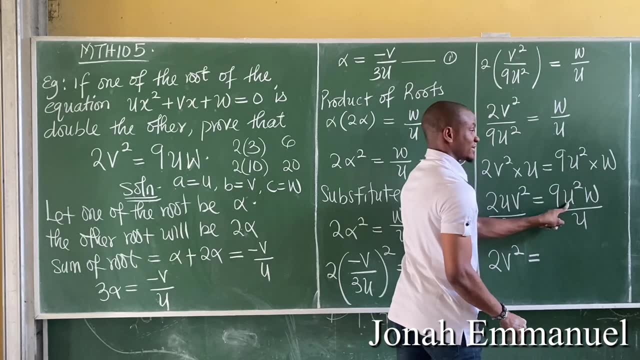 Divide here by u. This will cancel out. I'm having 2v. squared is equal to: Here is squared, Here is 1.. So this will cancel out one of it. I've left it. 9u. Bring down w. 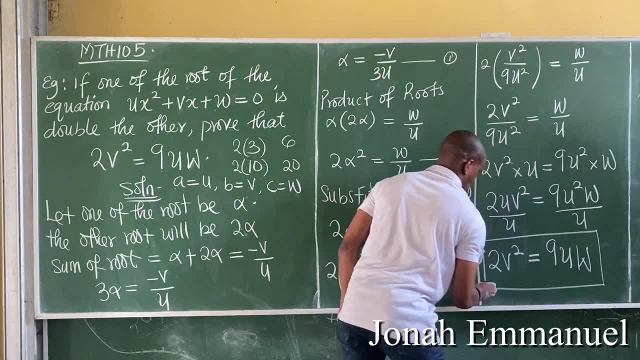 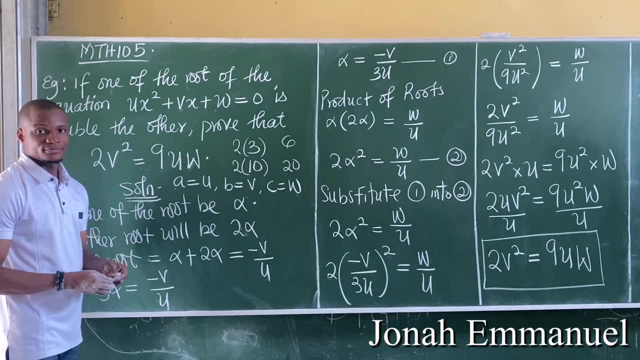 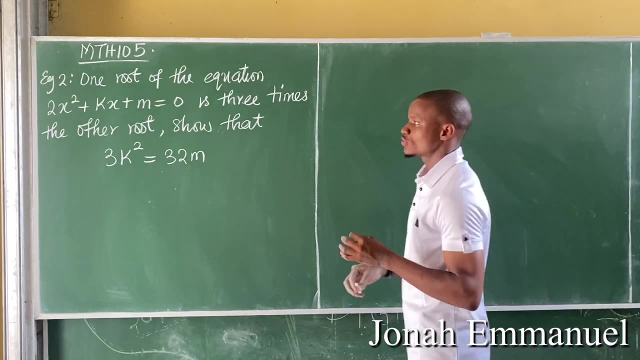 So this becomes the proof of what we have to do. So this is how we solve this. All right, So that's your proof of this. Let's look at a second example. We see one root of the equation: 2x squared plus kx plus n is equal to 0.. 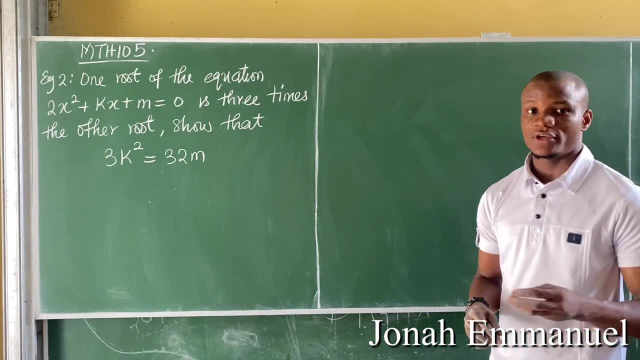 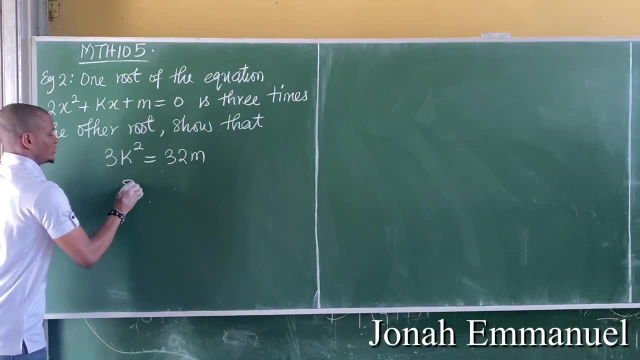 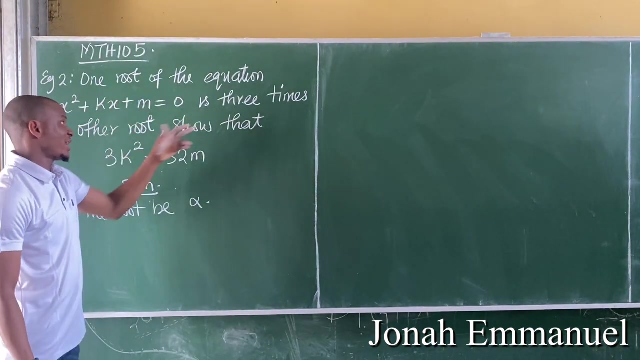 It is 3 times the order. Show that 3k squared is equal to 32f. How do you solve this? The solution Now we assume. We say let the root be or let one root be. what Alpha We said? one of the roots of the equation is 3 times the other root. 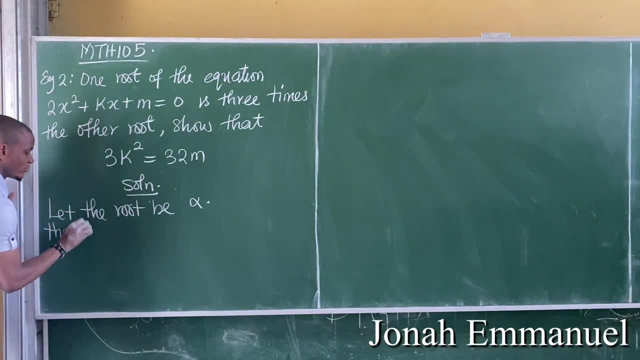 So if one of the roots is alpha, then the other root, which is 3 times the initial one, becomes 3 alpha. So my root becomes alpha and 3 alpha, 3 alpha. So my root becomes alpha because it's 3 times the other root. 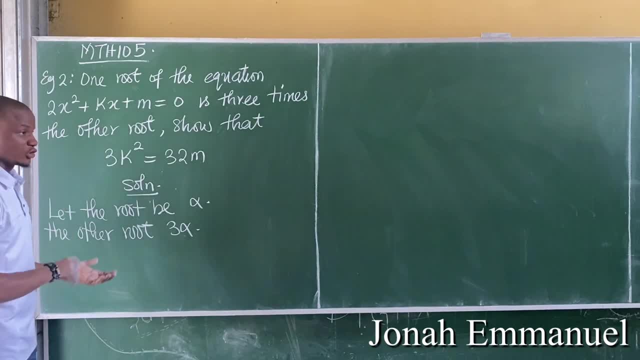 All right. So in this case, now Let's get some product of roots. So sum of roots, Sum of roots, is equal to sum this to: I have alpha plus 3 alpha, So it's equal to minus b all over a. 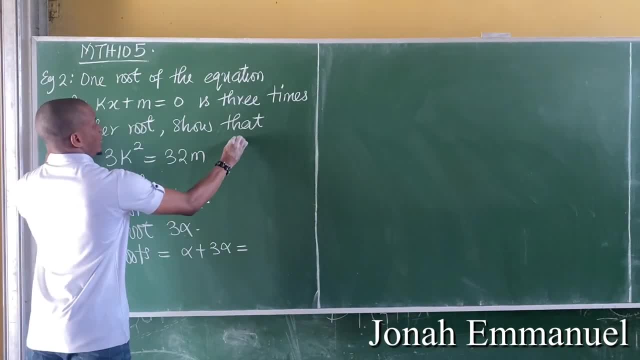 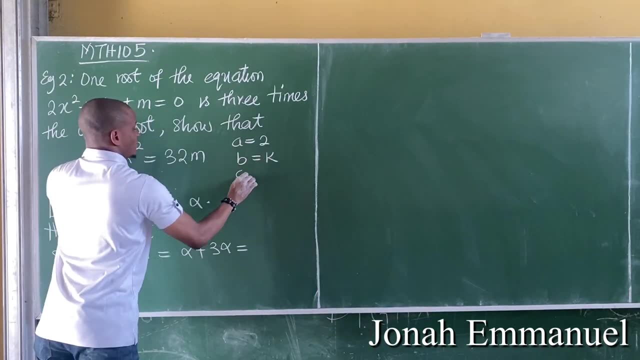 By the way, for this equation here, a is equal to this, which is 2.. b is equal to this, which is k, which is K, and C is equal to the constant, which is F. So if I have this now, equal to minus B, 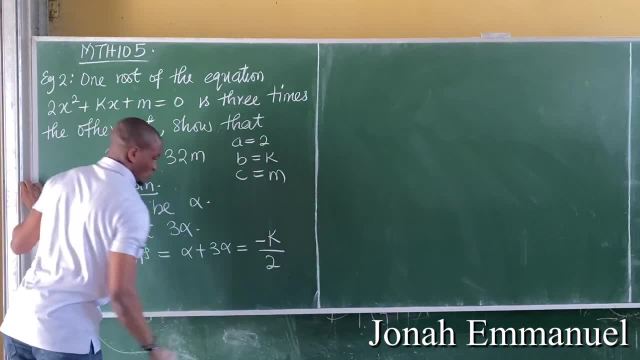 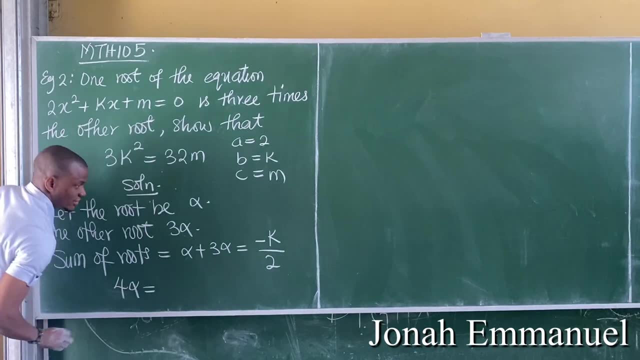 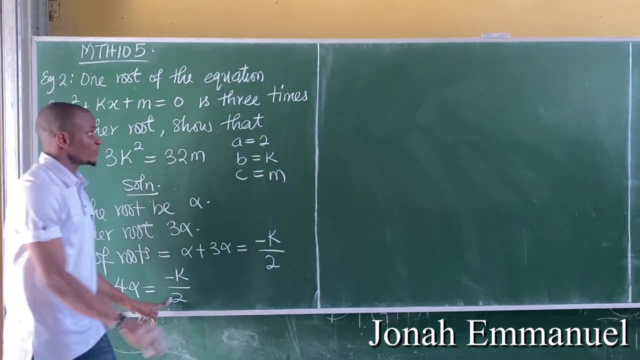 that's K all over A, which is two. So alpha plus three alpha gives four alpha, So four. alpha is equal to minus K all over two. Let's get the value of alpha. I'll move four over here. So it means that alpha is now equal to. 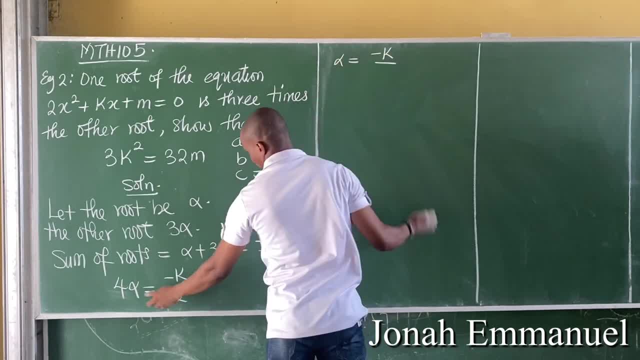 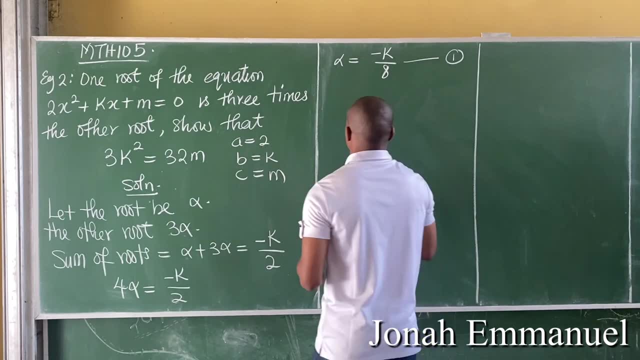 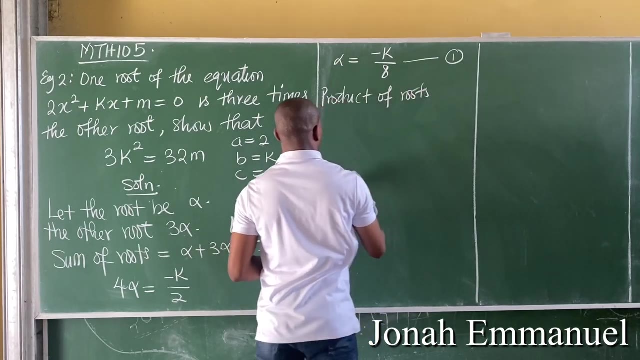 if I move four over here becomes minus K, all over four times two, that's eight. Call this the first equation. Let's now get product of roots. The product of roots now becomes: I'll be multiplying both roots If I multiply both roots. 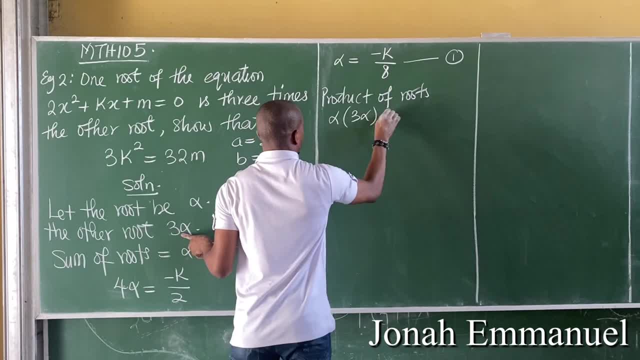 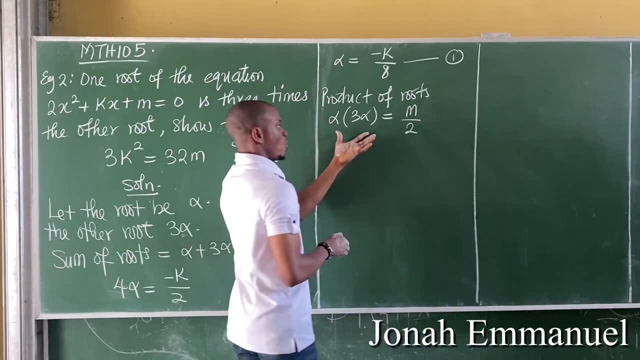 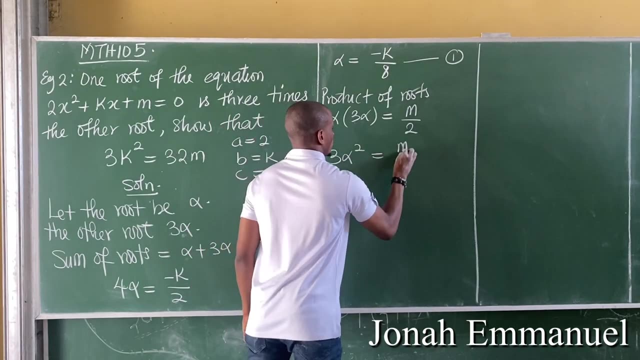 it becomes K Alpha multiplying three alpha, which is equal to C over A, That becomes N. all over A is two. So I have this. What this are? This gives three alpha times alpha gives three alpha squared is equal to N all over two. 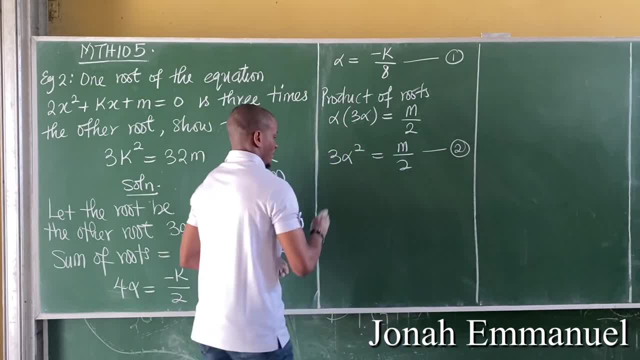 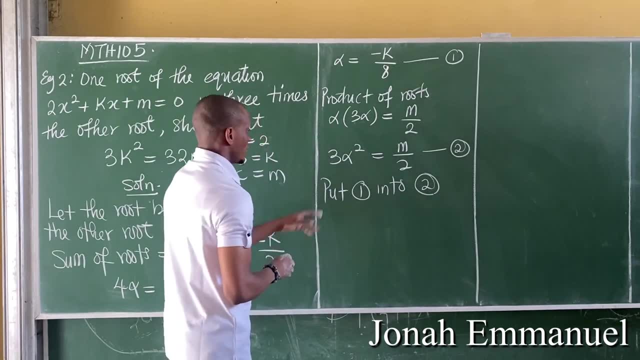 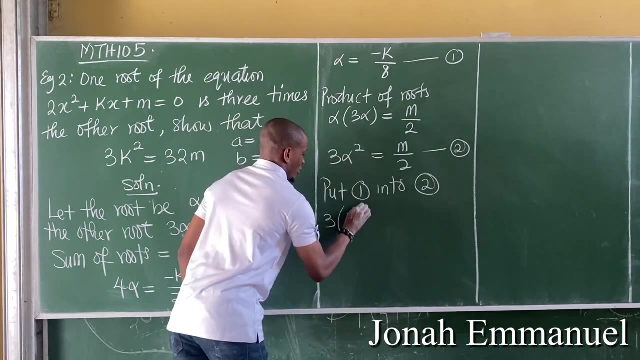 Call this the second equation. If I put equation one into equation two, what do I get? This becomes three into alpha squared. What's alpha? Alpha is minus K, all over eight, So three alpha squared is equal to N all over two. 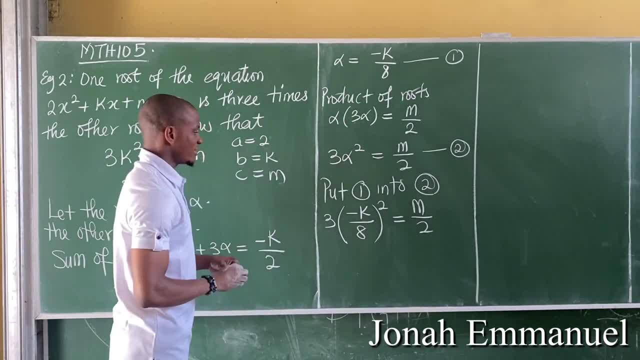 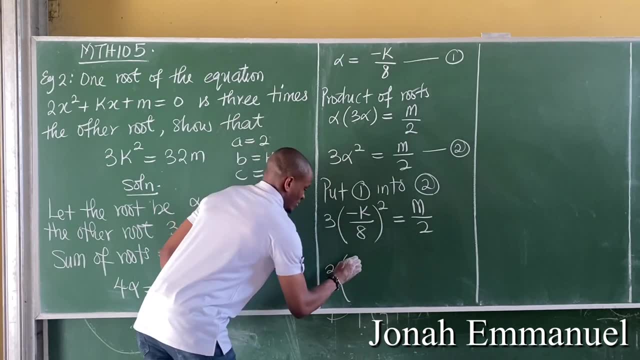 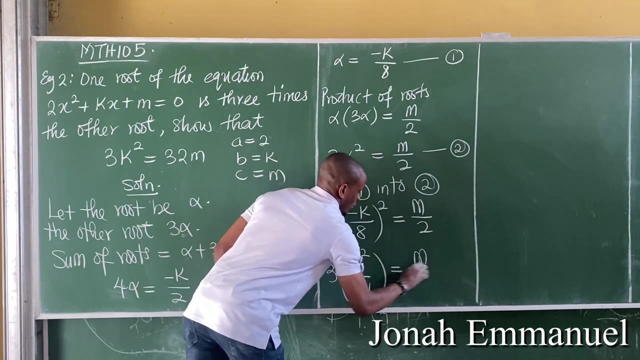 That's N all over two. What we solve. This gives three into minus squared, becomes positive K squared. So having K squared all over, eight squared is 64.. This gives three into minus squared, becomes positive K squared. This is equal to N all over two. 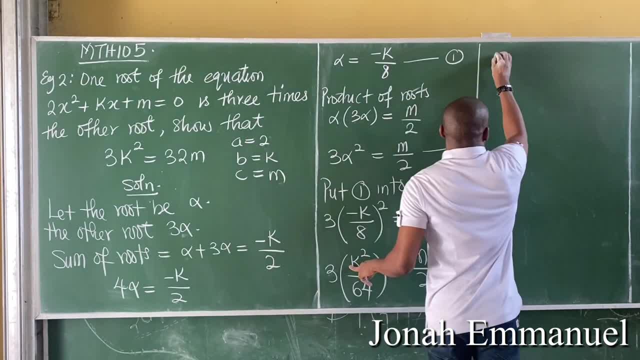 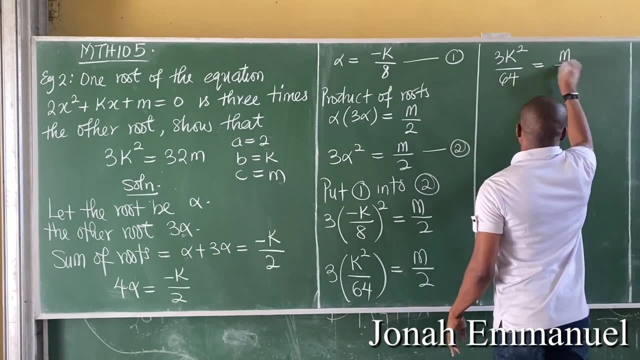 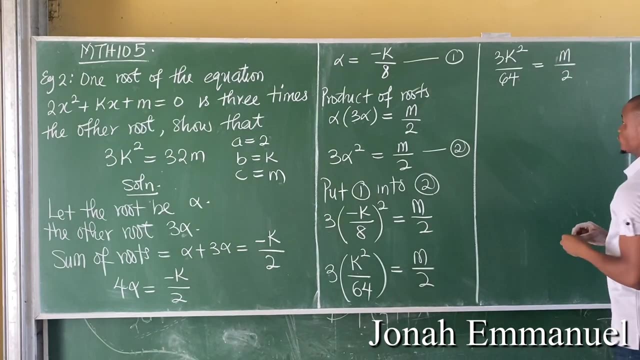 If I work this out now, three multiplies here, that is three K squared all over this, 64 is equal to N over two. So I have this: Simply move 64 over here. Or you can say: cross, multiply it one, two. 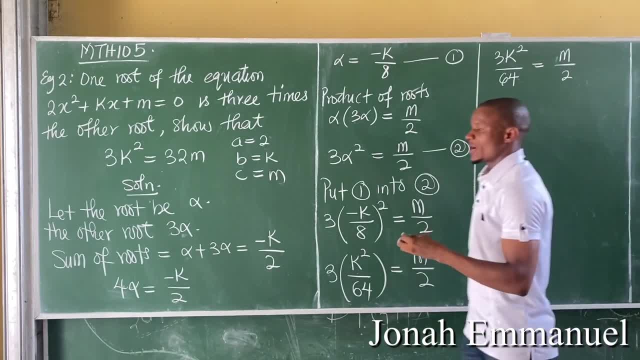 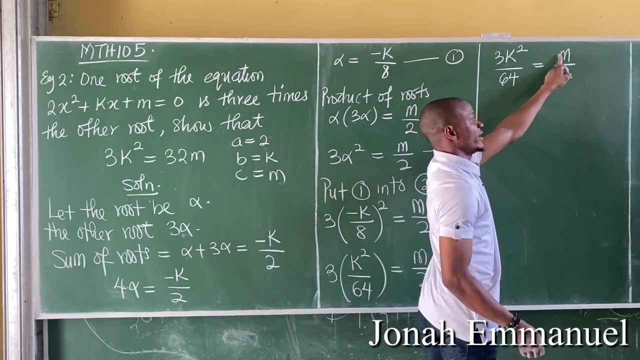 But I think it's easier if you move it all over here, Right? Remember, we are asked to prove three K squared, right? So we've already have three K squared. now. It's better if you leave it here Instead. it goes all over here. 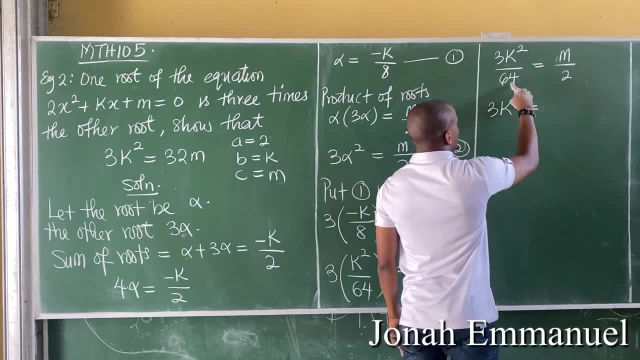 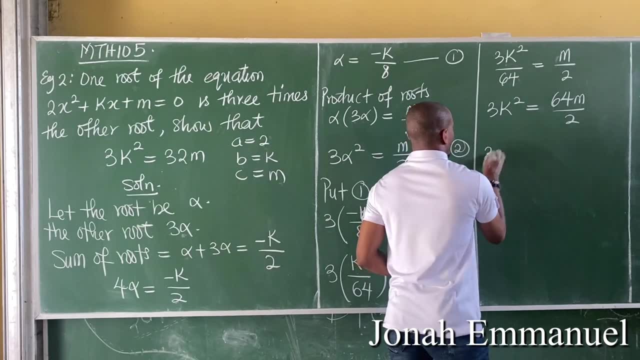 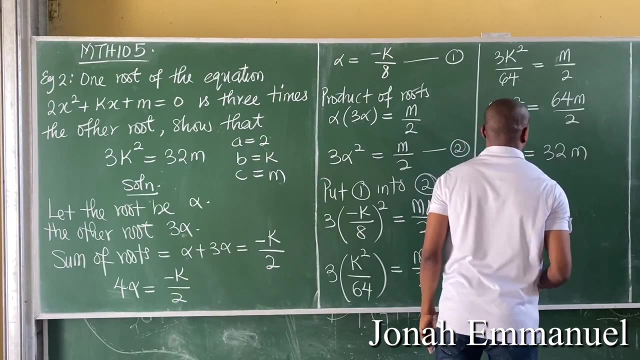 So I'll have that three K squared is equal to 64, comes this way, becomes 64N all over two. What we solve This is: three K squared is equal to 64, divided by two Gives you 32N. So this becomes the proof of what we are asked to find. 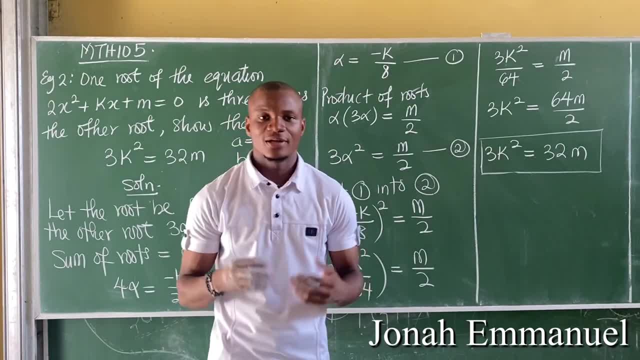 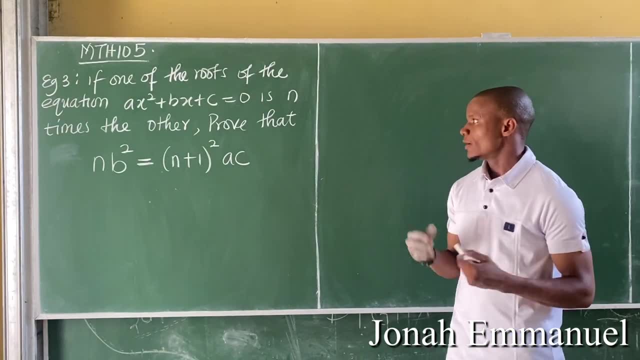 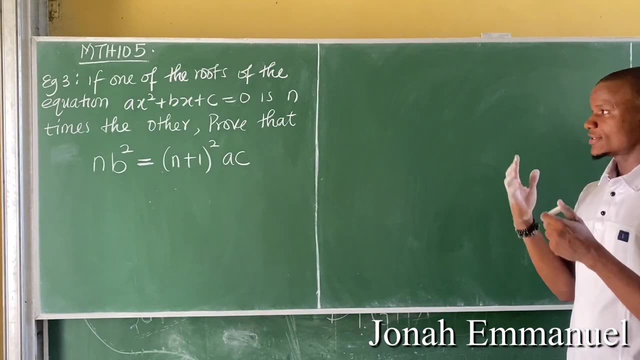 So it has been proven. So this is how we solve problems like this. All right, So let's look at one last example of these kind of problems. Okay, It says: if one of the roots of the equation, AX squared plus BX plus C is equal to zero, 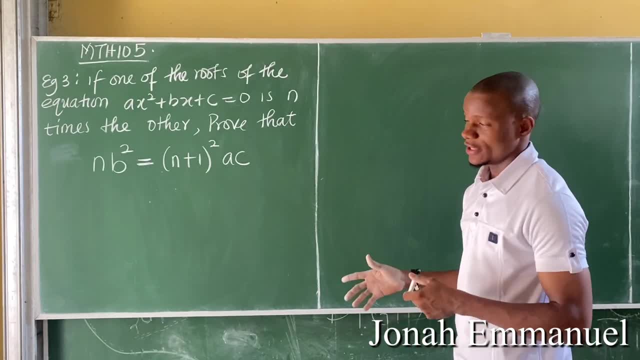 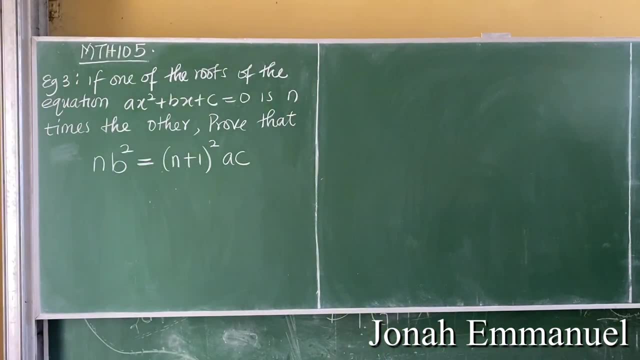 is N or it's N times the order. All right, It's N times the order. Come on, Prove that N is squared. The answer is: A is squared, All right. so let's look at one last example on this kind of problem. 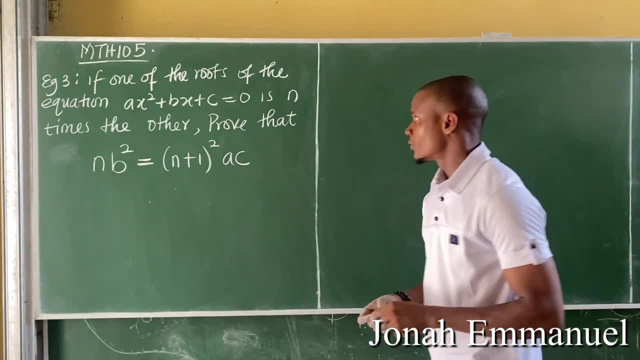 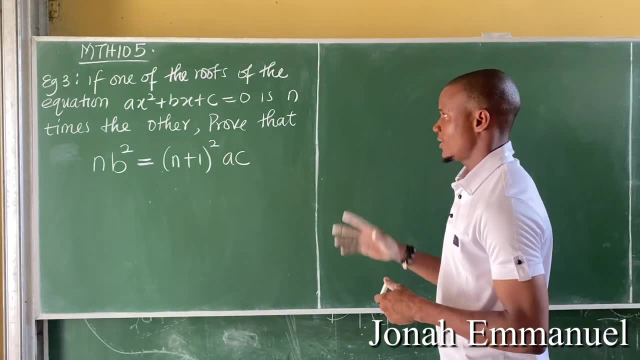 It says: if one of the roots of the equation, AX squared plus BX plus C is equal to zero, is N times the order proof that NB squared is equal to N plus one, all squared AC. All right, So how do we work on this? 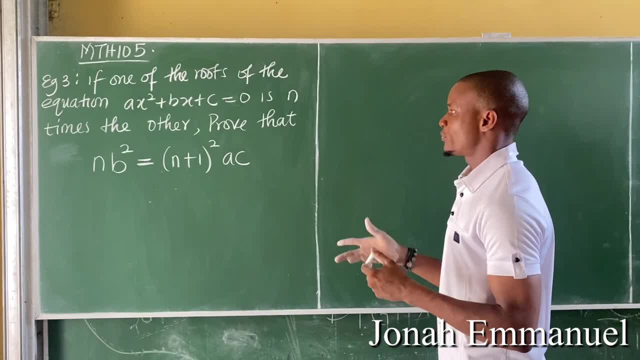 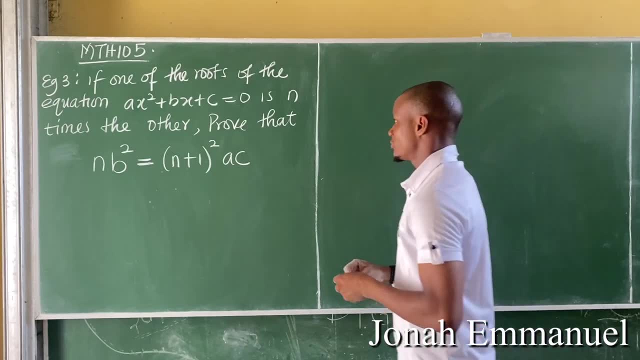 See N times. the order Prove that NB squared is equal to N plus one all squared AC. All right, So how do we work on this? So for the simple problem, that is, we look at the depreciation, we look at the depreciation. 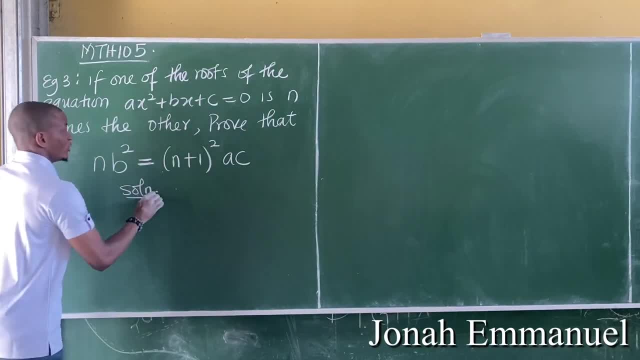 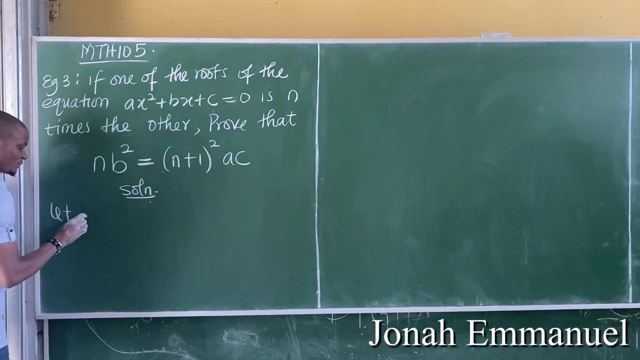 easy Summation. Of course this is general method or general form of a quadratic equation. So here A is A, B is B, and then of course C is C. So let's assume, So let's let one. 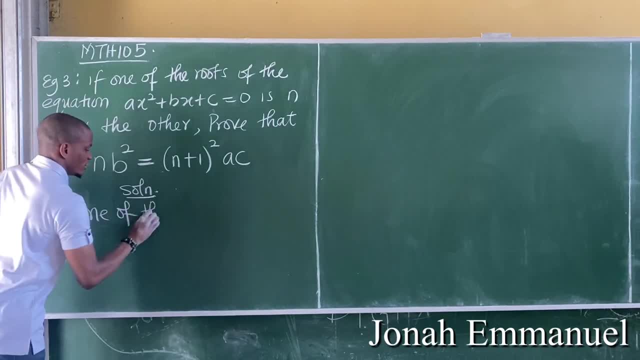 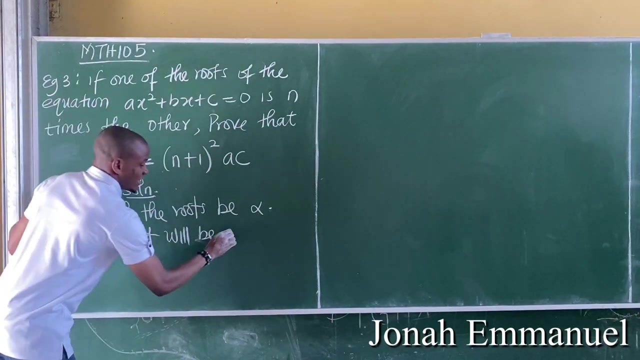 of the roots. let one of the roots be what? The alpha, The alpha, The other root. the other root will be: the set is N times the other. alright, So it becomes N times. this one here will be N alpha. So if one is alpha, 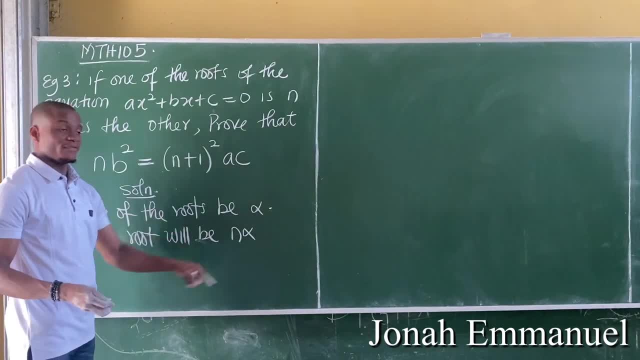 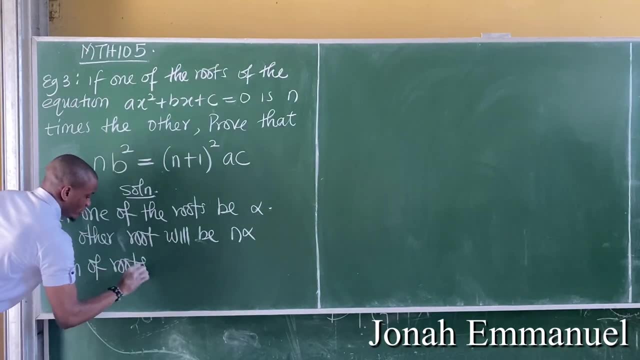 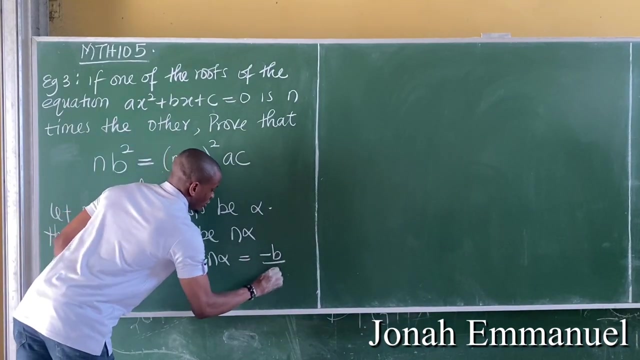 The other one becomes N times alpha. That becomes N alpha. alright, Let's get sum of roots. So sum of roots, the sum of the roots will be given by alpha plus N alpha. okay, And of course that becomes equal to sum of roots. equal to minus B under A. I could. 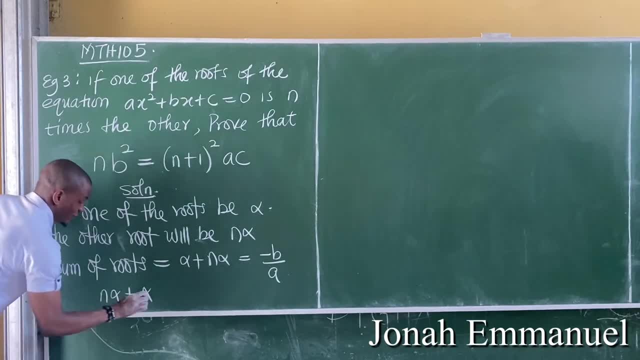 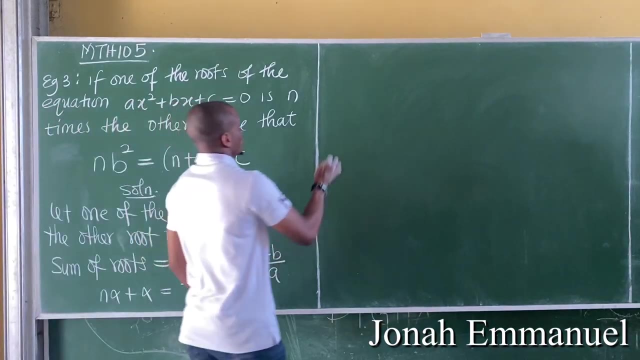 write it as saying N alpha plus alpha, They are the same thing. So this is now equal to minus B all over A. Of course, obviously, these two cannot add up, but I can still factorize it. I'm seeing alpha, I'm seeing alpha, So 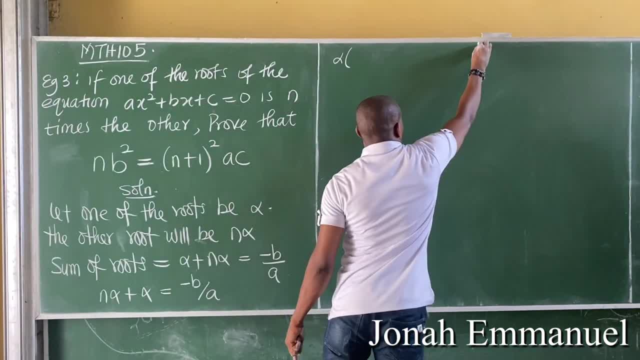 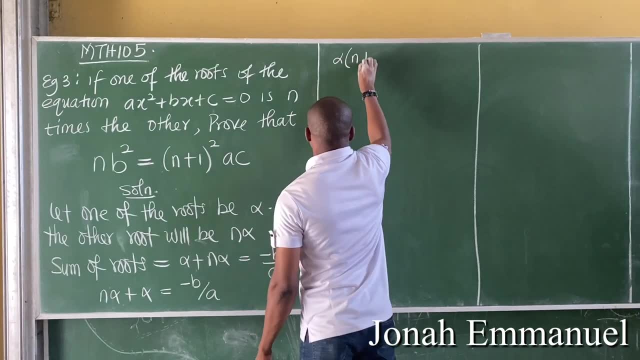 take out alpha. If I take out alpha, divide N alpha by alpha, alpha comes out. I'm left with N. plus divide alpha by alpha: I'm left with 1, is equal to. I'm left with N. I'm left. 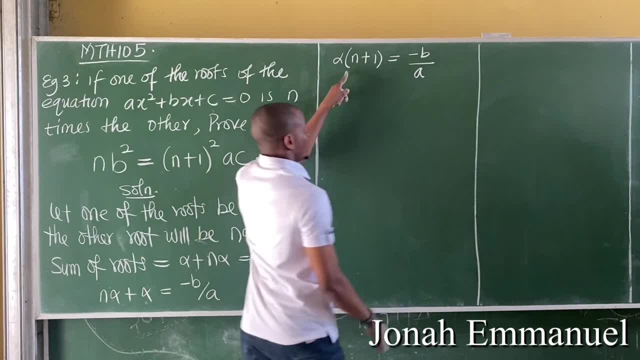 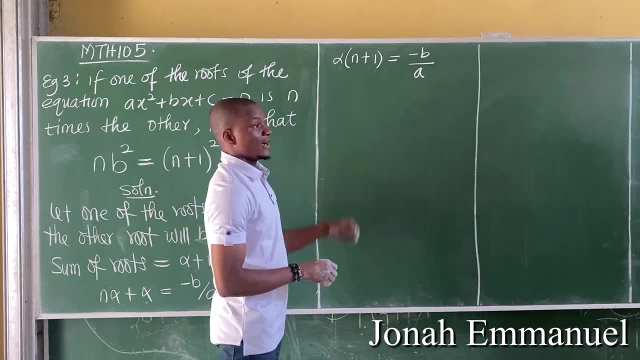 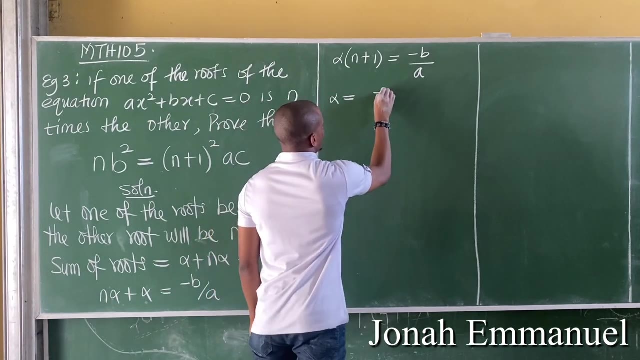 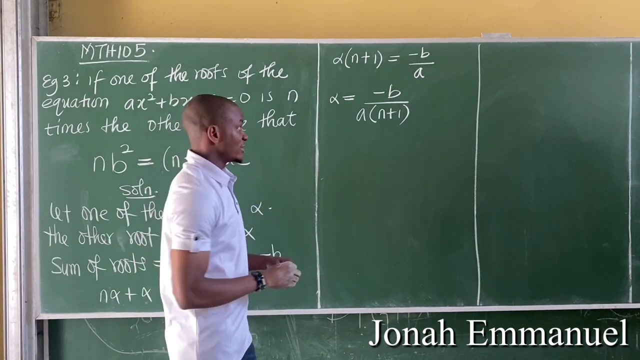 with N plus minus B all over A. So I'm having: alpha into N plus 1 is equal to minus B over A. Let's make alpha subject of the formula. How Divide the sign by this. So I have that alpha is equal to minus B all over A into N plus 1.. So I have this Alright. 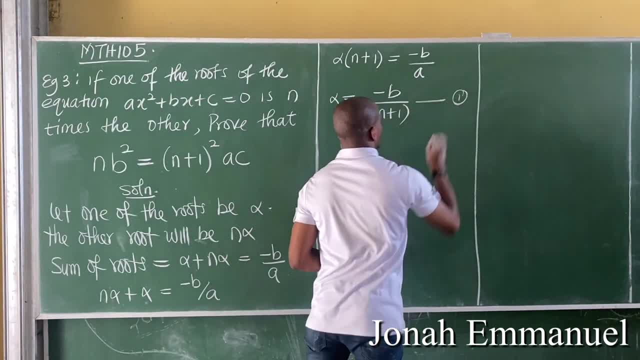 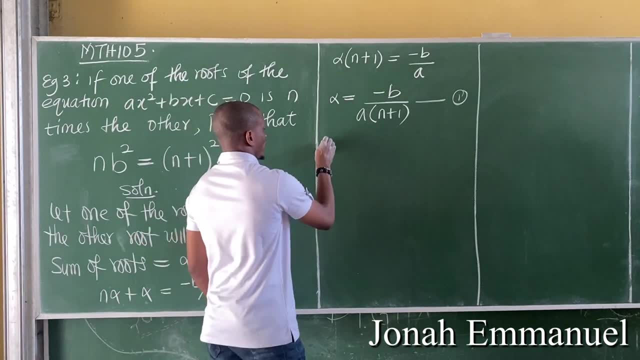 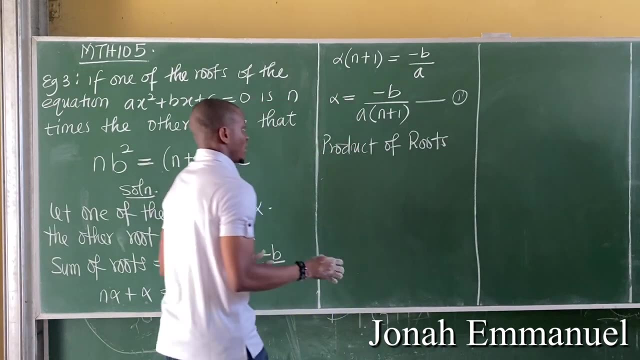 so we can call this our first equation, perhaps Equation 1.. Let's now get the product of roots From here. the product of roots, that would mean I'm multiplying these two, So it becomes alpha, multiplying the second root. 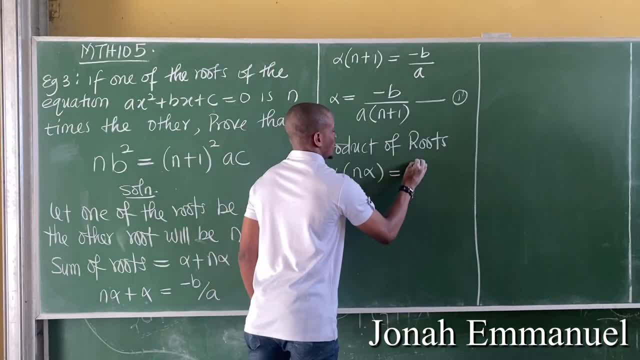 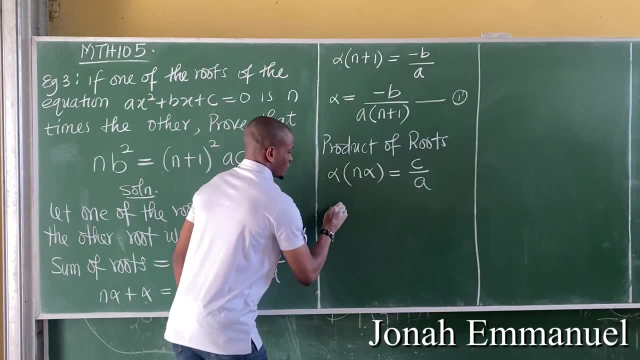 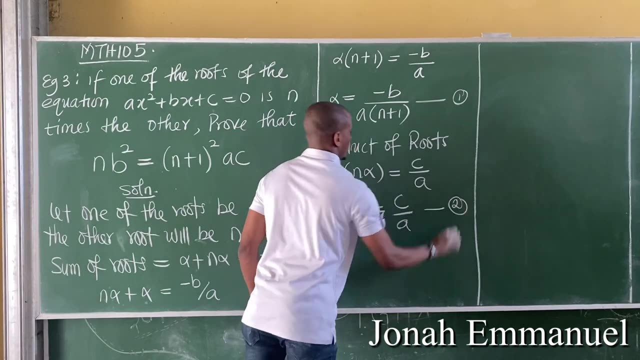 N alpha into N alpha, which is equal to C over A for product of roots. If I multiply this this time, this gives you N alpha. N alpha squared is equal to C over A. Call this your second equation. If I put equation 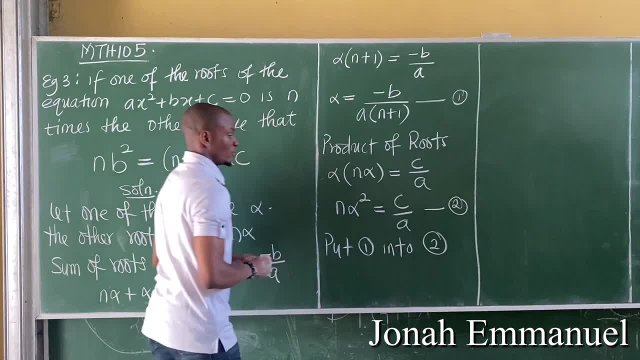 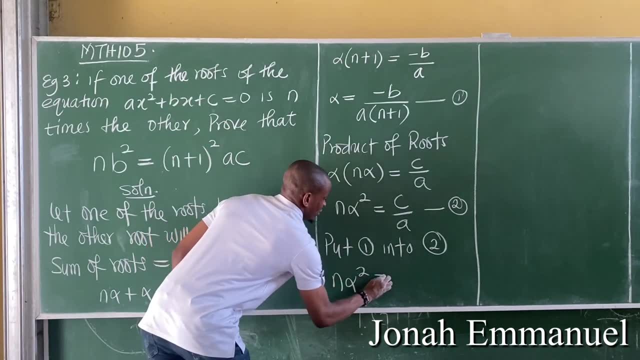 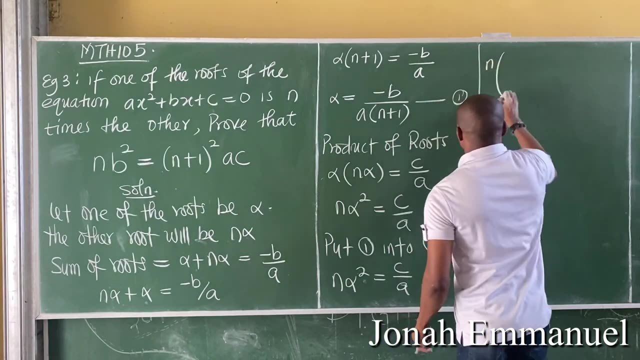 1 into equation 2, see this now becomes equation 2. says N? alpha squared is equal to C over A. So see the body of alpha. this now becomes N? A2, alpha is minus B all over A. So this: 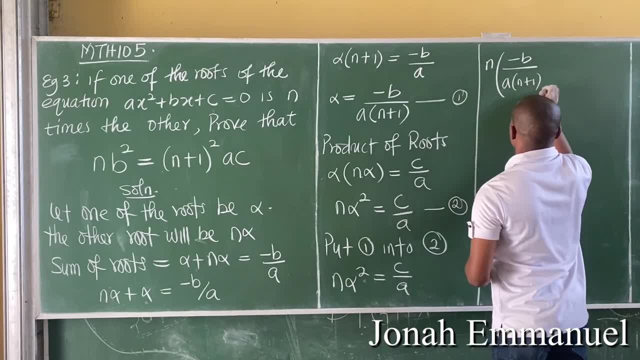 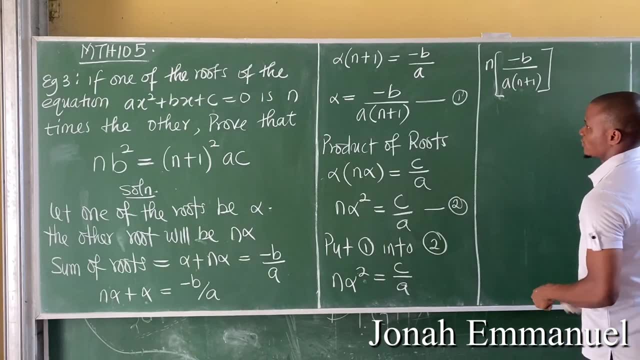 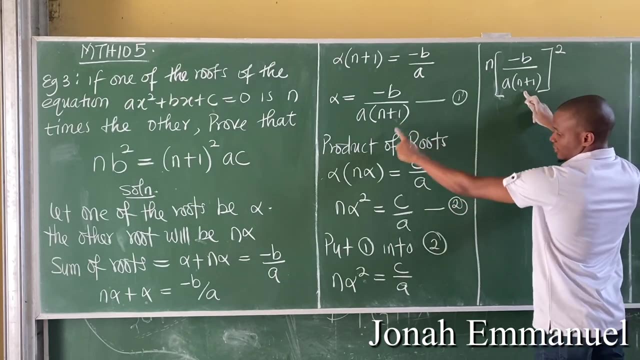 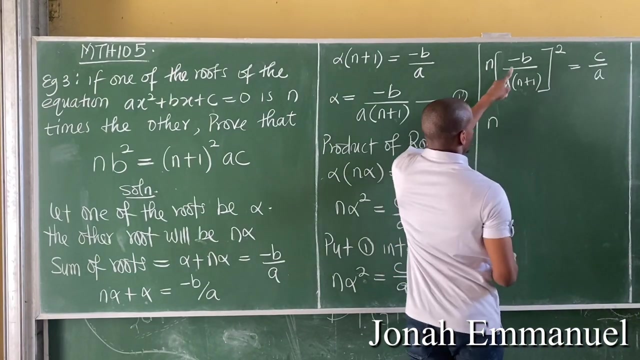 is A into N plus 1.. Perhaps it's better I use a square bracket here, Since I already have a round bracket. I'm using a square bracket. So N into alpha squared Here is alpha. Okay, that's this. All squared is equal to C over A. What this is this is N into minus squared. 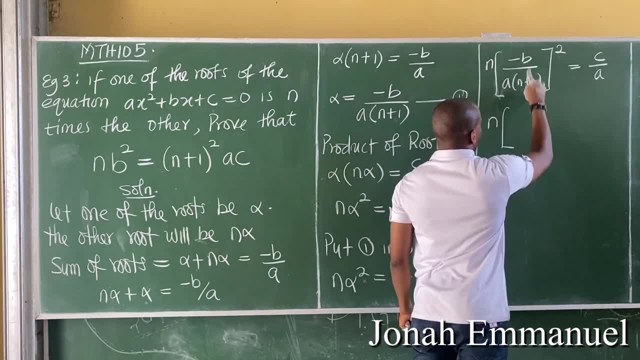 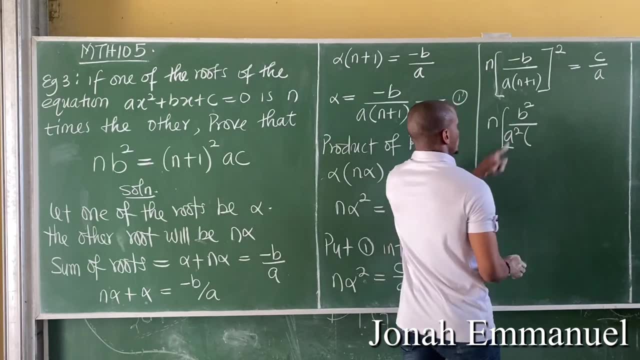 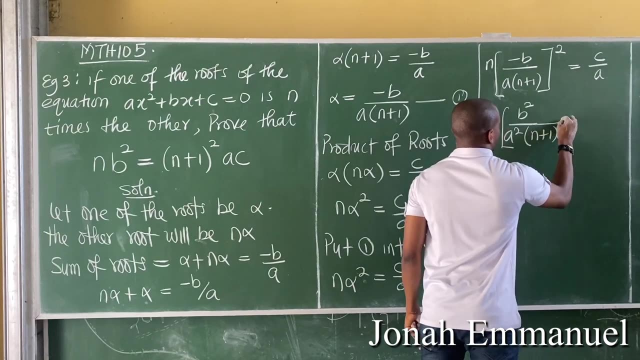 becomes positive, into B squared, That's B squared all over A squared, That's A squared into this one here squared, That's N plus 1 all squared. So I'll get this an expansion, I'll get: this is equal to C all. 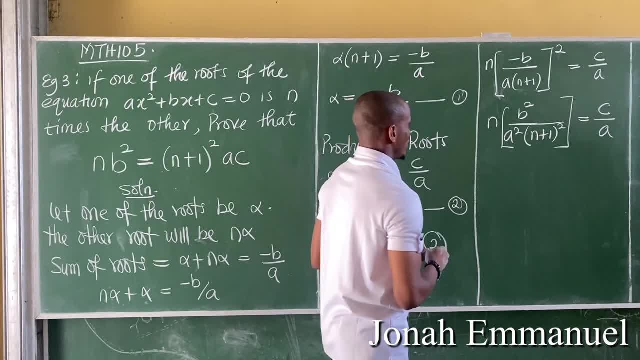 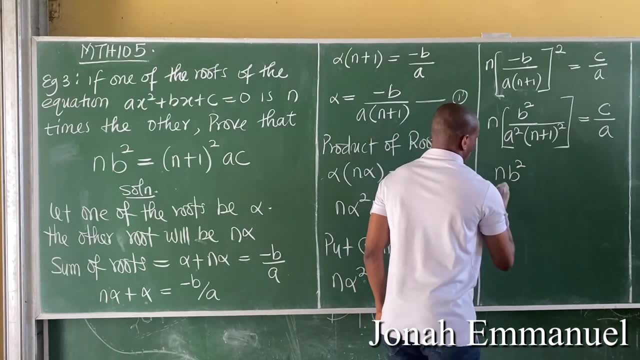 over A, So I have this All right. so what we saw now, this one line is: I have this line is: I have N B squared all over A, So I have this All right. so what we saw now. 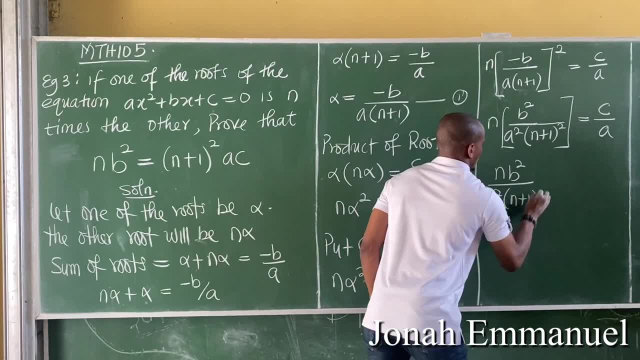 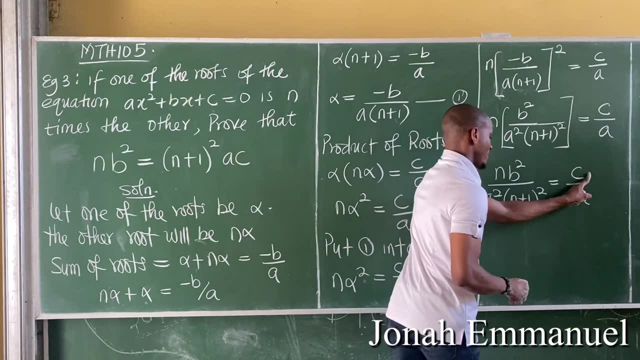 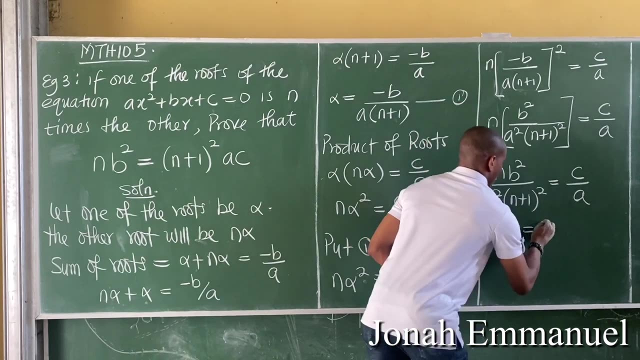 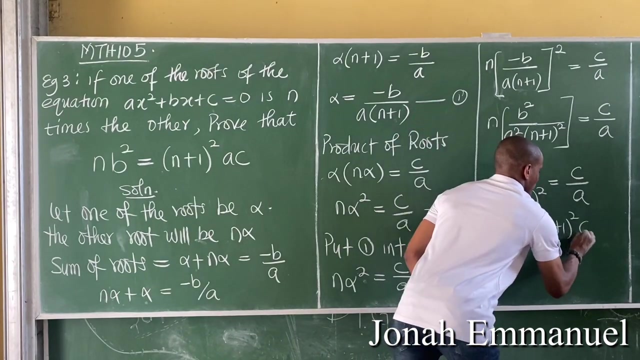 A squared into N plus 1, all squared is equal to C all over A. My next task will be move this one over here, So I'll have that N B squared is equal to this. one comes here, becomes N plus 1 all squared. So take this one first. This one goes here, becomes A. 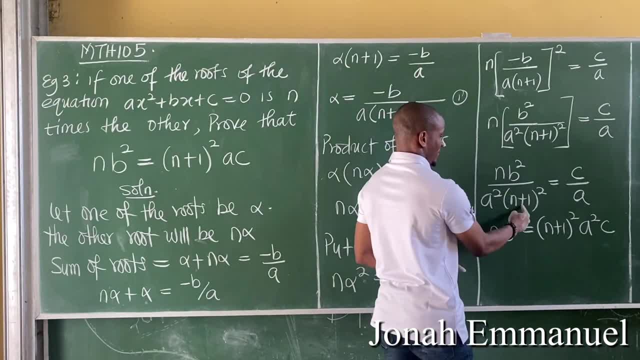 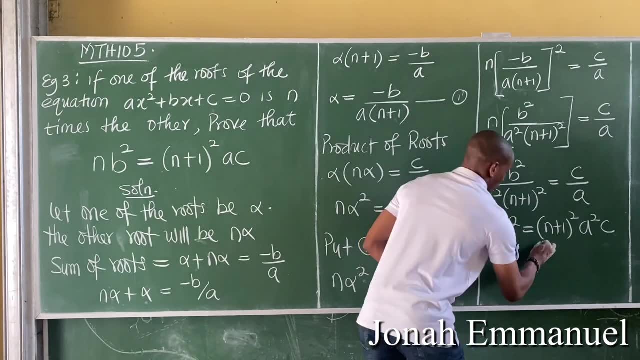 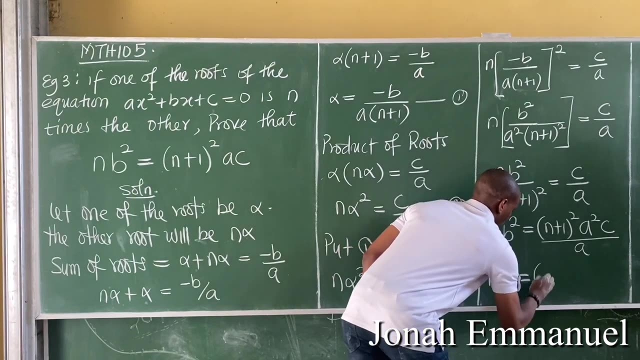 squared times C. All right, So N plus 1 squared A squared times C. These two are multiplied. I'm just rearranging it here. All right, All over what there A. So this now becomes N. B squared is equal to N plus 1 all squared. 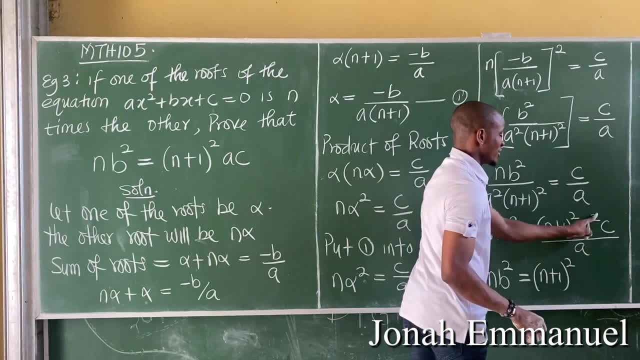 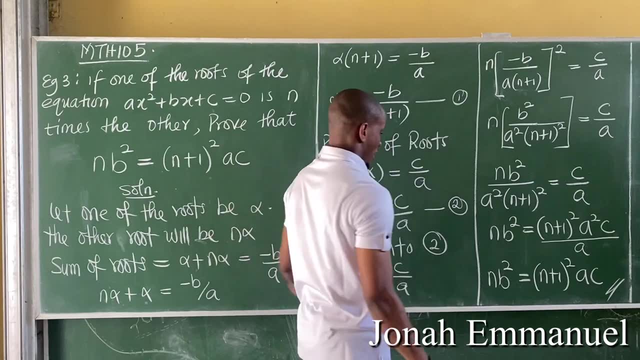 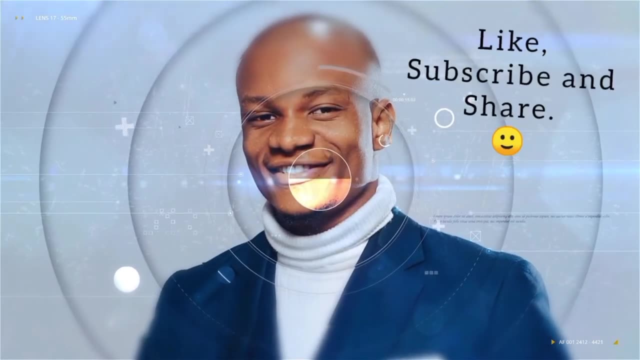 Of course A. this is A squared A. there will pass one A, It becomes A and then C. So this is the proof of what we are asking. All right, So this is how you solve this Problem. 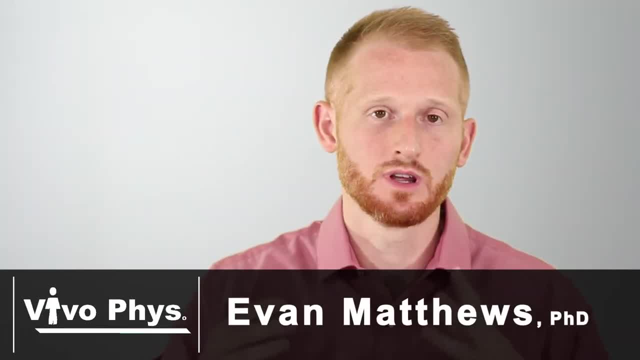 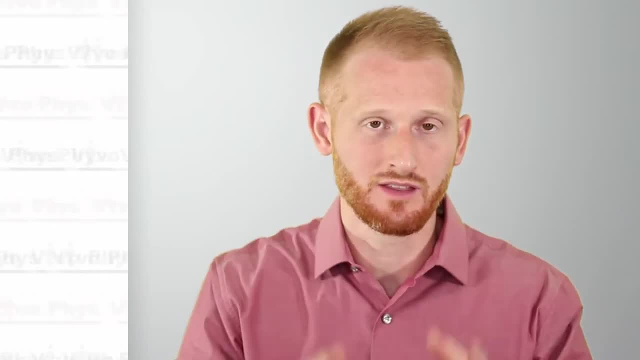 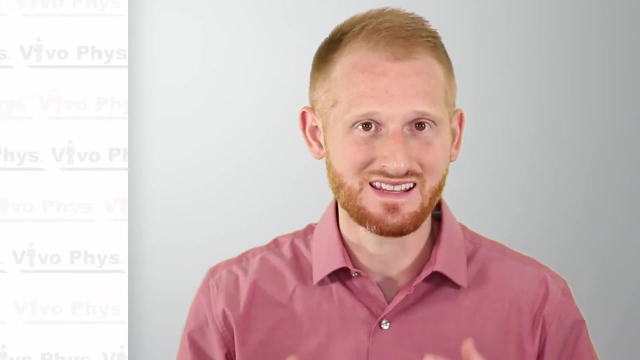 Let's show an easy way of looking for outliers within your data. So you really do want to look at all your data points individually and within the columns, so within the variable and sort of, scrutinize each one the best of your ability, but you need to have a starting point. 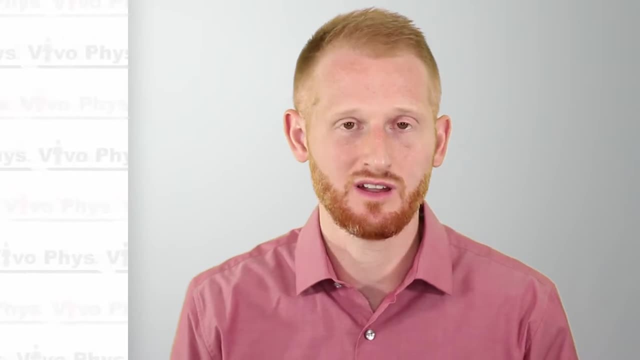 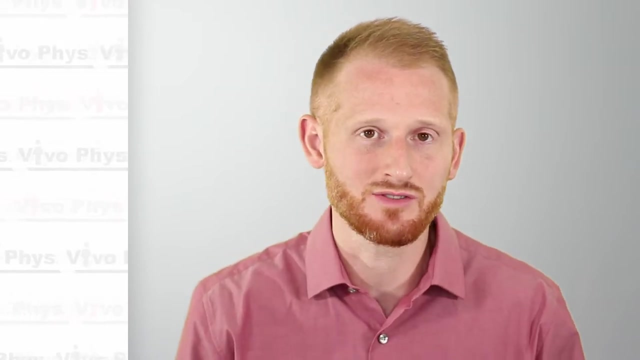 of way of doing this. Looking at the minimum and maximum values can be helpful, but it's not very objective and especially if you're looking at numbers that are fairly abstract and you're not as familiar with yet, it might not be all that helpful. So what we can do: 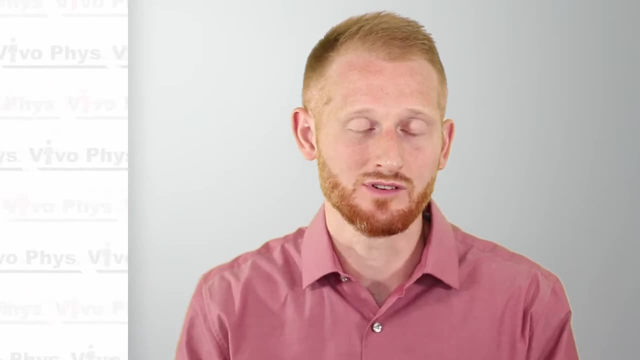 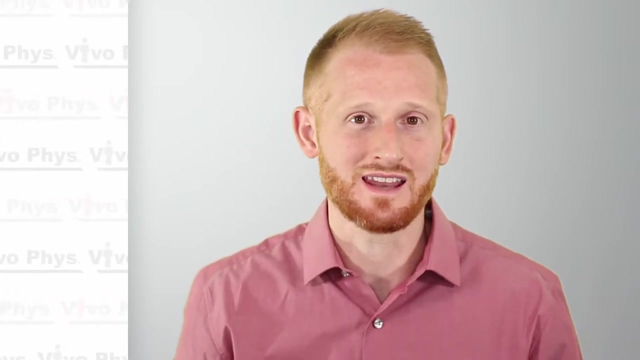 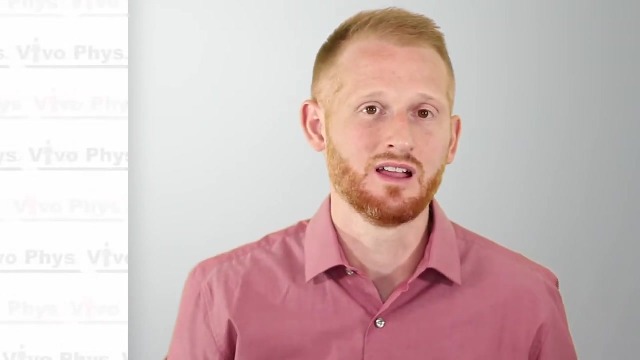 is, calculate how far away from the average the minimum and maximum values are and use that to help us determine if there is potentially an outlier, whether it's an outlier because there's some sort of typo or error in the database, or it could be a physiological outlier where it's real. 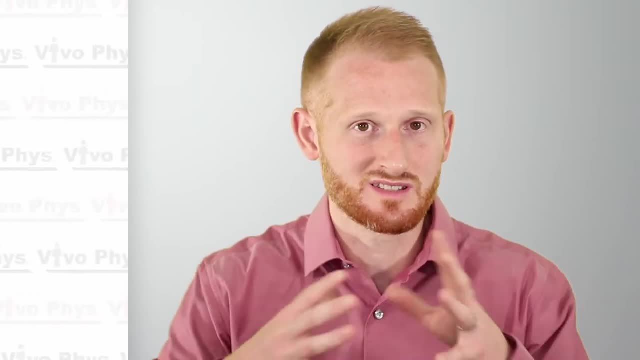 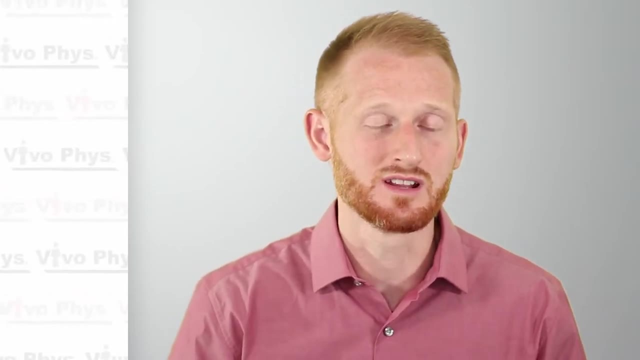 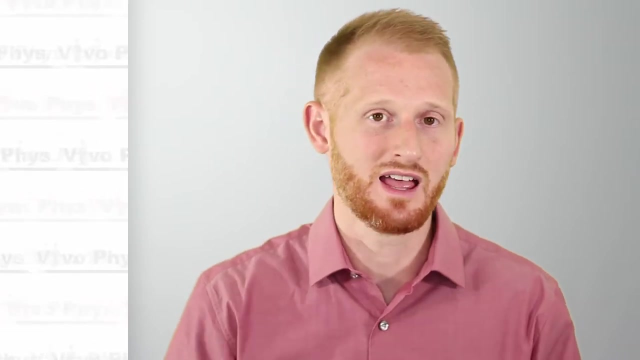 data but the person was just a little atypical. So in a small data set one atypical person can really throw off the whole data set. So they might be somebody you might want to consider not using within your data. Of course there's a lot of sort of should I or shouldn't I not throw? 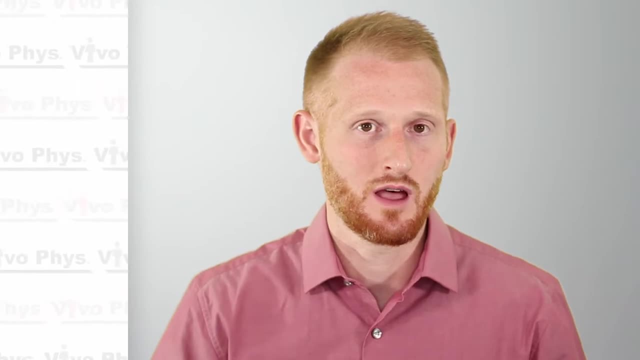 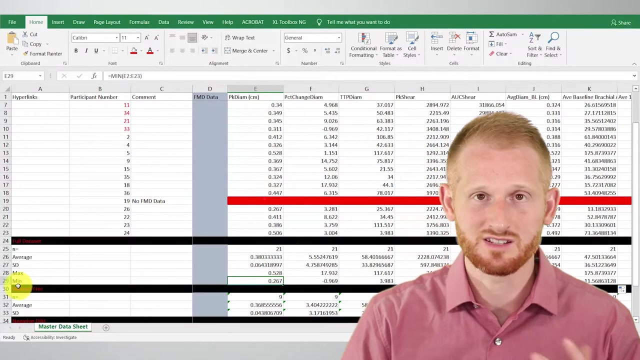 out outliers. It's going to come up to you and your biostatistician to determine if that's something you should do or not, But let's go ahead and show how we can identify potential outliers this way. So I'm going to insert a row here. 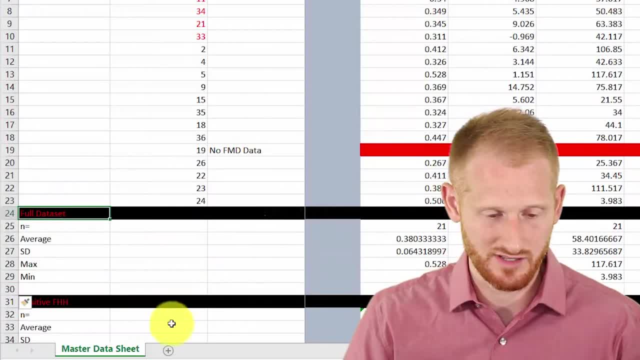 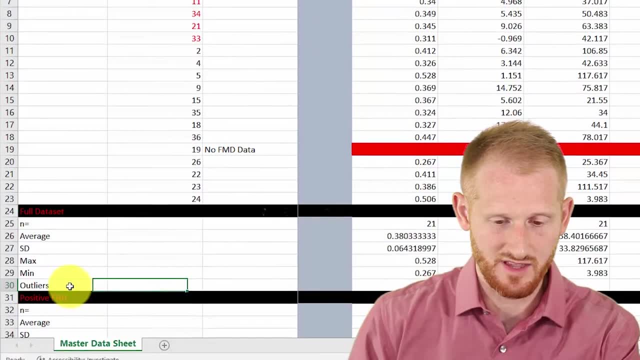 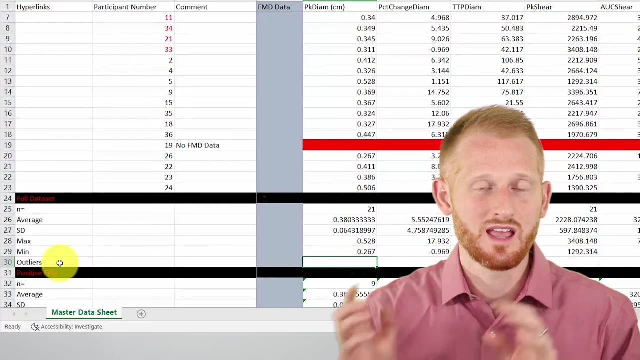 in our full data set area of our statistics And let's type in outliers. Alright, so this is going to be a formula that I'm going to have you go to the description of this video, copy the formula and paste it in, just like I am doing, And I'll show you then how to modify it to fit your, your.